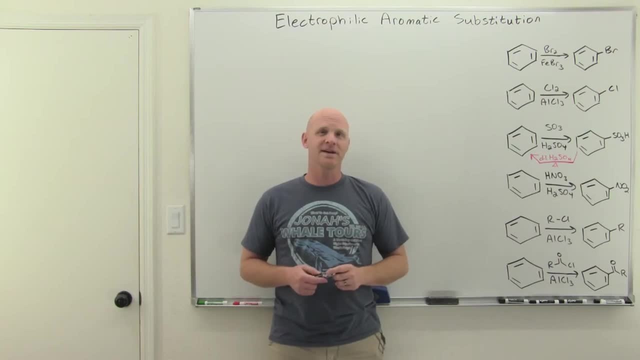 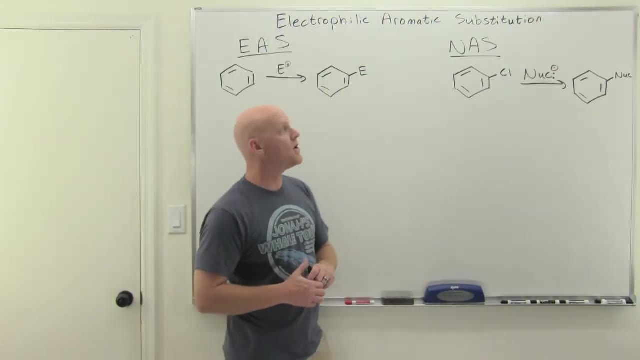 every time I post a new one, subscribe to the channel and click the bell notification. All right, so before we dive headlong into electrophilic aromatic substitution, I just want to do a little compare and contrast here with electrophilic aromatic substitution. 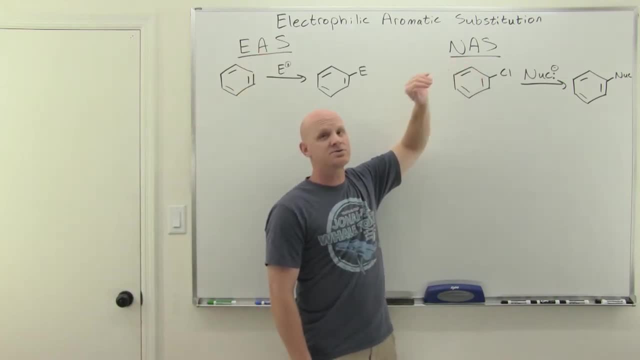 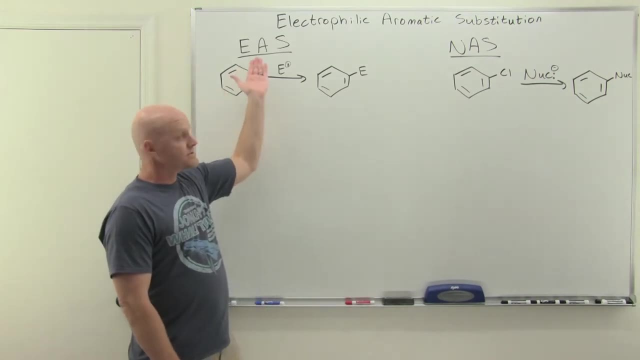 Substitution, or EAS for short, and nucleophilic aromatic substitution, or NAS for short. that we'll cover at the end of the chapter, just so we see the difference up front before going on here. So in electrophilic aromatic substitution we are going to be substituting a hydrogen, that's 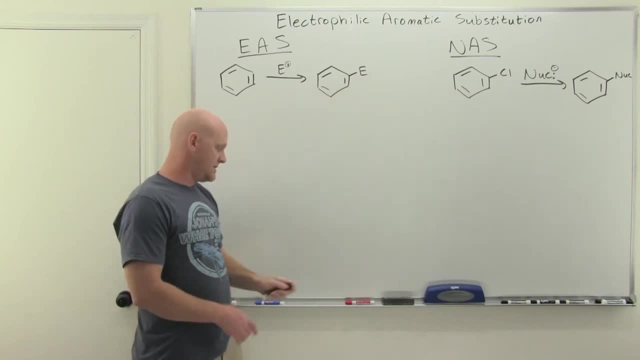 on the original benzene here with an electrophile, And so in this case, if benzene is reacting with an electrophile, well that means that benzene must be acting as the nucleophile, and that will be important later on. Now, in nucleophilic aromatic substitution we are going to be substituting a 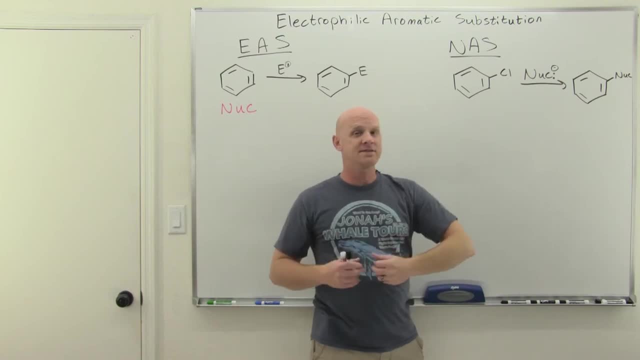 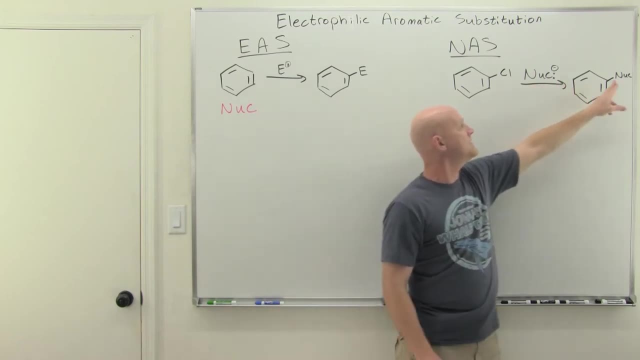 nucleophilic aromatic substitution. We're not replacing a hydrogen. We'll be replacing what we would have thought of as a traditional leaving group, a halogen like chlorine or bromine- It's pretty typical- And we're replacing it with a nucleophile. So when we call it nucleophilic, 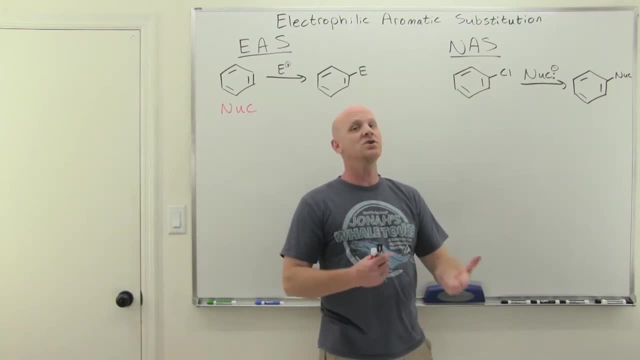 aromatic substitution. it's that we're substituting a leaving group here with a nucleophile. Now again, if benzene here is reacting with a nucleophile, well then benzene must be acting as the electrophile, And this will be some fundamental differences between EAS and NAS. 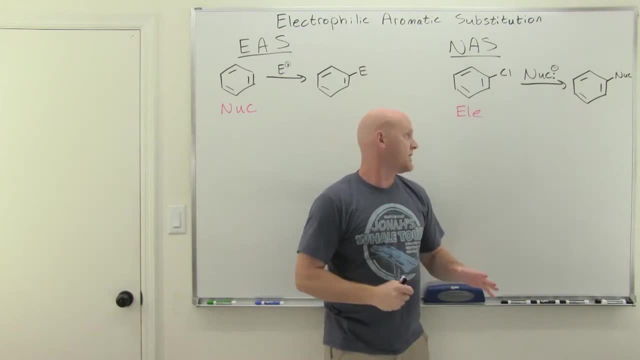 that will point out the difference. So we're going to be substituting a nucleophile here with an electrophilic aromatic substitution that will point out later on. Cool. So now that we kind of got that out of the way, let's talk about the general mechanism in electrophilic aromatic. 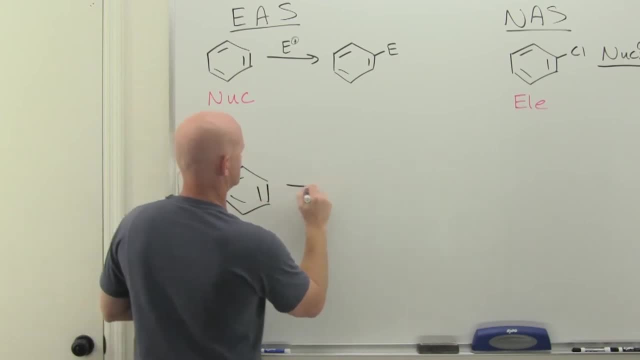 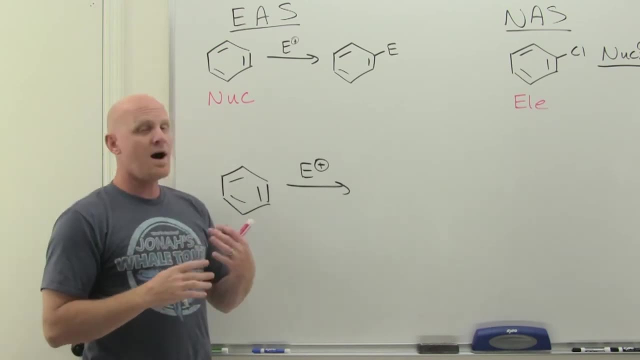 substitution. Okay, so the general mechanism is actually pretty simple. It's just two steps. What's going to make this more complicated, though, is that benzene is not the most reactive thing And, being aromatic, it's very stable. The electrons are very low in energy, And so, for this, 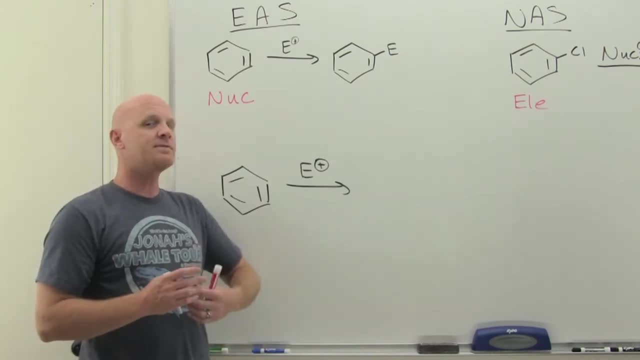 to work you have to have an amazing electrophile, And amazing electrophiles just don't sit around on the shelf for very long, So you have to make them in C2.. And so we mix reagents that will first react to create this electrophile, And then we can kind of do the standard EAS reaction. So the way 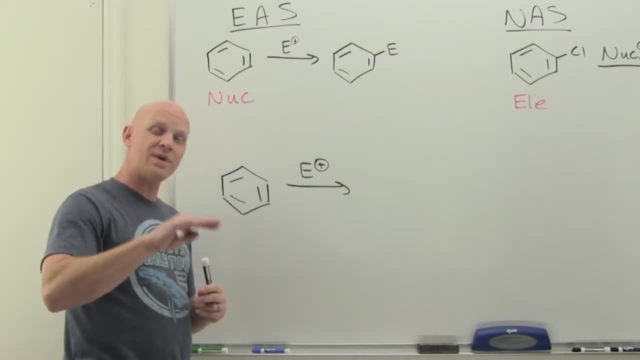 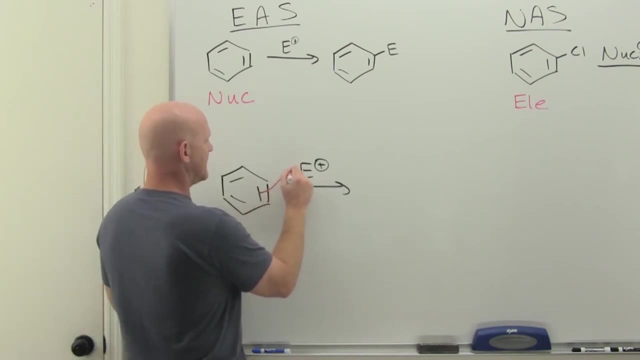 this works once you actually have your electrophile generated and all the individual reactions have a different, a little bit different way in which that electrophile gets generated. So once you have it, then first step is nucleophilic attack. So your benzene is going to come and attack that. 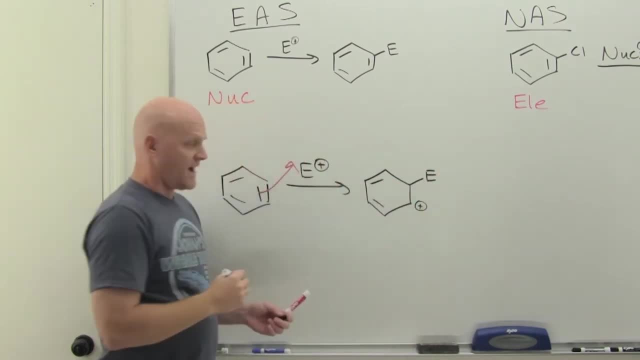 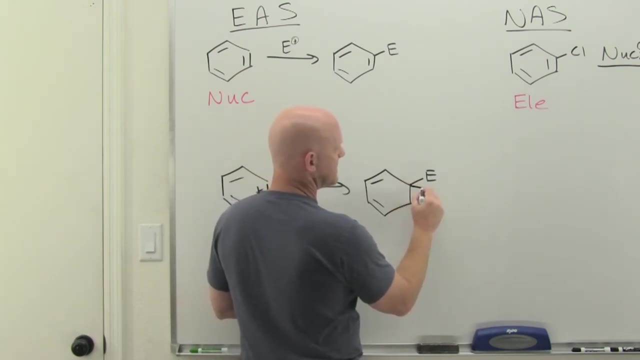 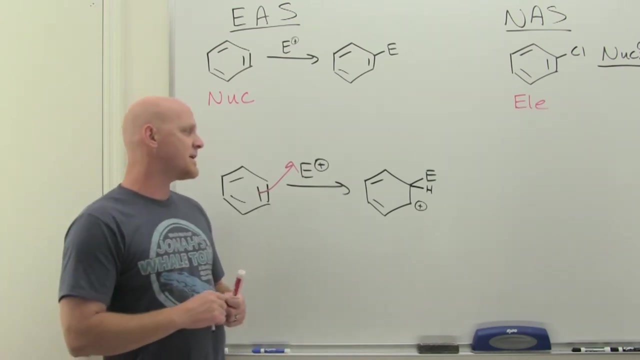 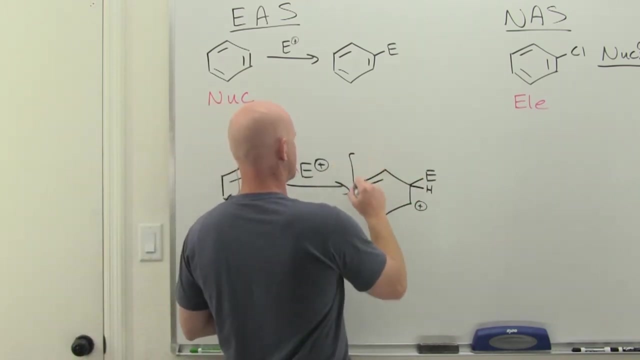 we'd like. So, as you can see here, if you remember, I actually had a lot of up, but I'm going to try to do it a little bit more quickly. So first you put in a little bit of the eosin and you put in a little bit of the phenylphthaleate, Which is actually in the most liked way of the reactor. So we're going to take a little bit of that And we're just going to put in a little bit of the hyaluronic acid. So then we're going to put in a little bit of the boson, So that's the last thing that we put in there. 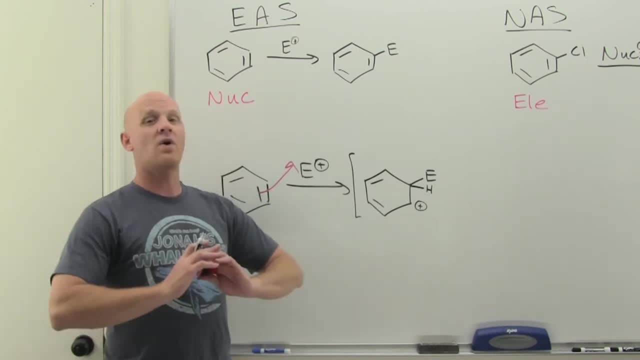 So it's going to get it in the first place, and then we have to get it back together, So I'm going to all these resonance structures often makes this looks more complicated than it is, So I'm going to wait for a second. Now, had this just been a regular alkene, like, let's just say, we take those. 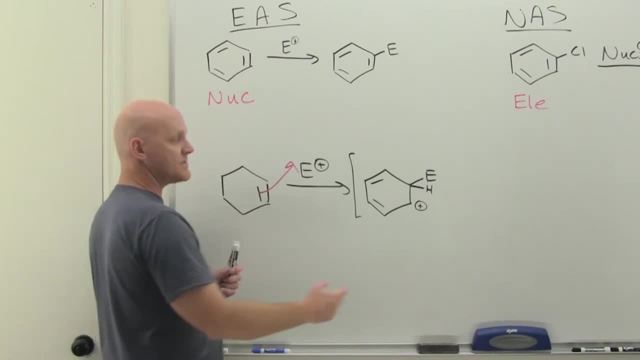 off for a second. then we'd add the- you know electrophile to one side and then we'd have a nucleophile coming back and attaching right here And we would just do addition instead. So but big thing here is that we've got an aromatic ring. If we do addition, we're going to end up. 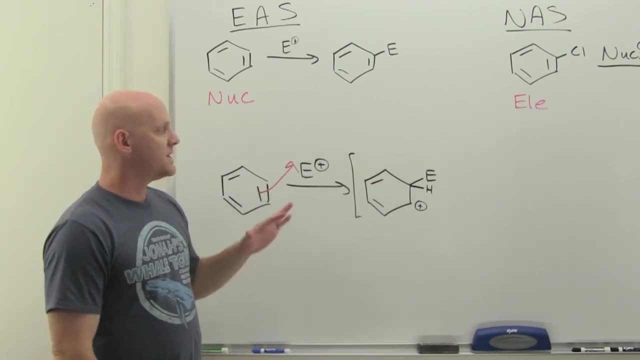 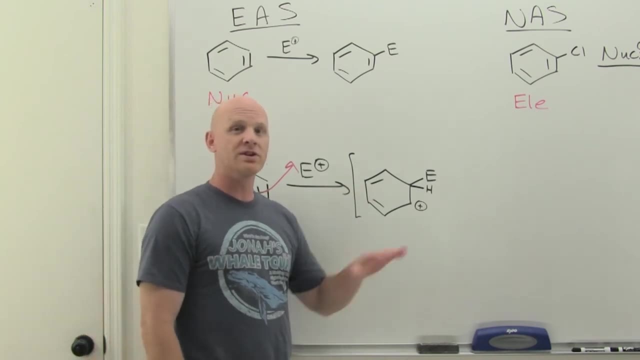 with a final result of something that is not aromatic, Whereas if we eliminate this hydrogen to restore aromaticity, we'll end up with a much more favorable and lower energy product instead. So in this case, that's why we're going to do substitution instead of addition, because we 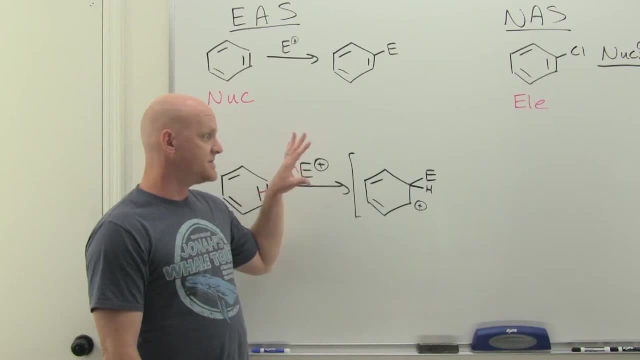 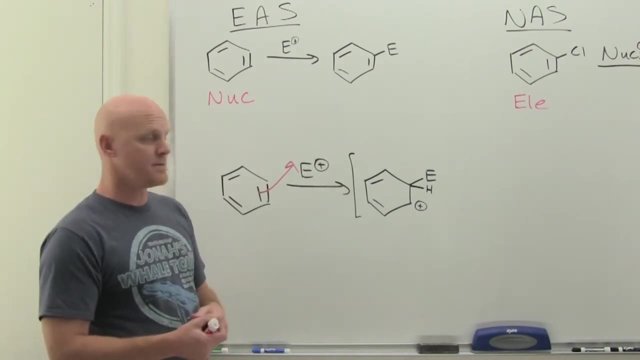 end up with an aromatic product and it's much more energetically favorable. Addition largely is not going to occur in these reactions in any sort of real competition. It's all going to go through this electrophilic aromatic substitution. So in this case we're going to have some sort of 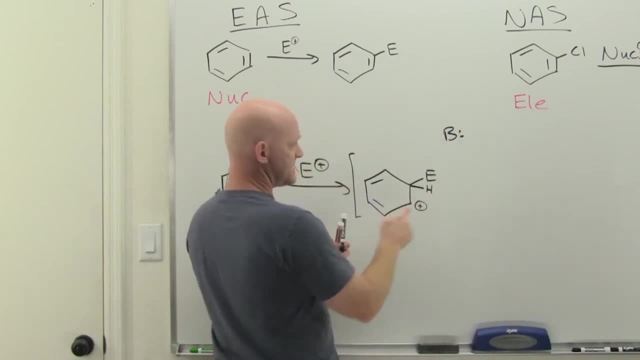 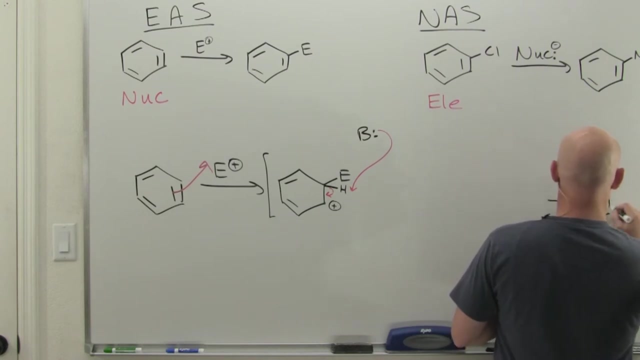 base coming along, So and that base is just going to come and deprotonate here, So and that frees up these electrons to become pi electrons and restore aromaticity to the ring, And so in the end we complete our substitution there. So again, I did say that we're gonna have 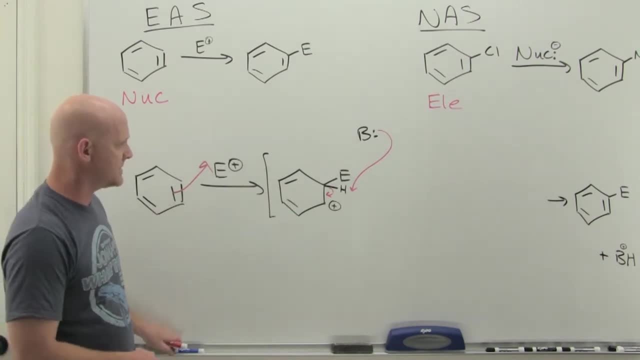 to show some resonant structures And so this carbocation is definitely resonance stabilized And so we're going to have to show some resonance structures And so this carbocation is definitely resonance stabilized And so if we show some resonant structures here, we could move these. 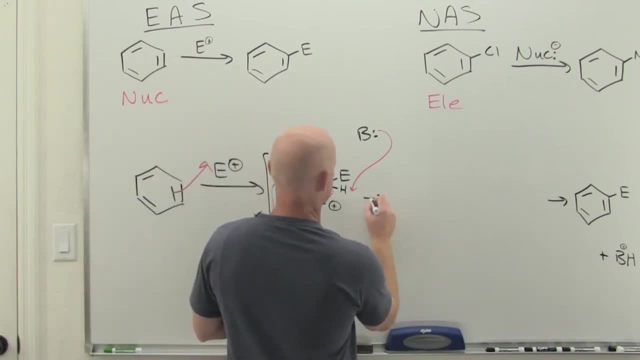 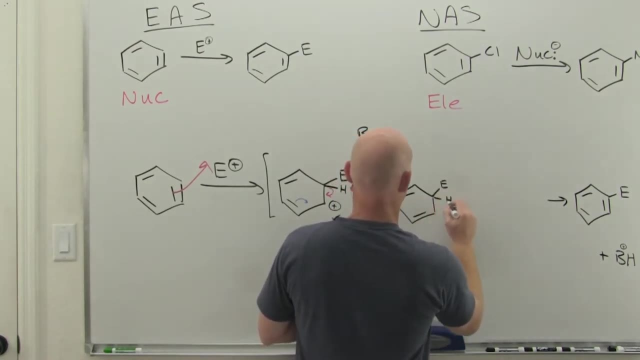 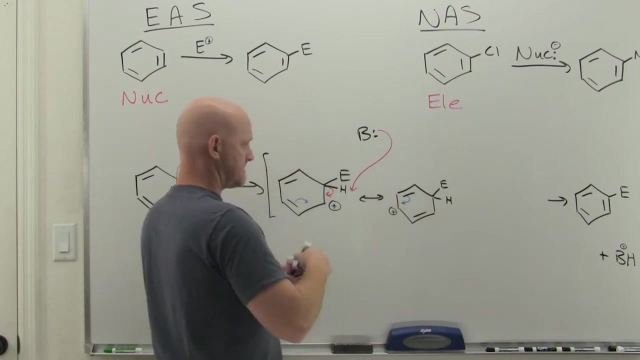 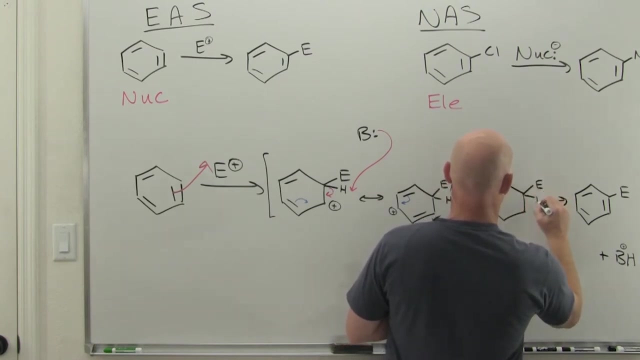 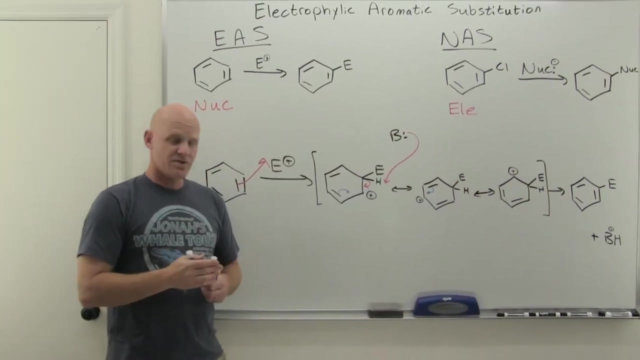 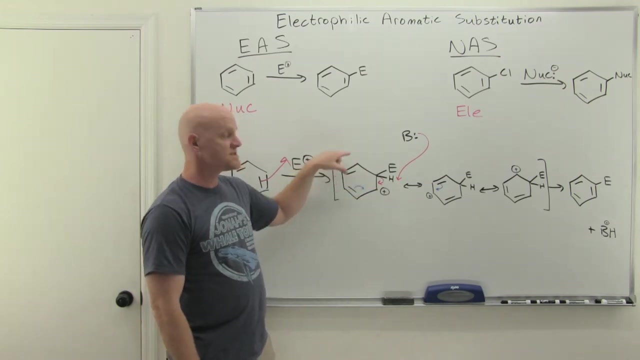 electrons here Puts the positive charge here And once again that's one bond away from these pi electrons So we can move them here. Cool. And so that positive charge is in principle going to be shared on three locations on the benzene ring. So we'll find out that if we have some substituents attached, so preferably in one. 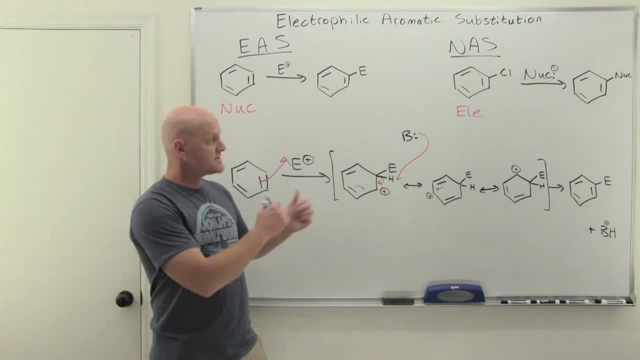 of these three locations, we'll find out. it can have profound impacts And even, in some cases, add additional resonance structures beyond this and make this even more stable. Or in other cases, we'll find out that other groups you might have attached actually might make this lovely. 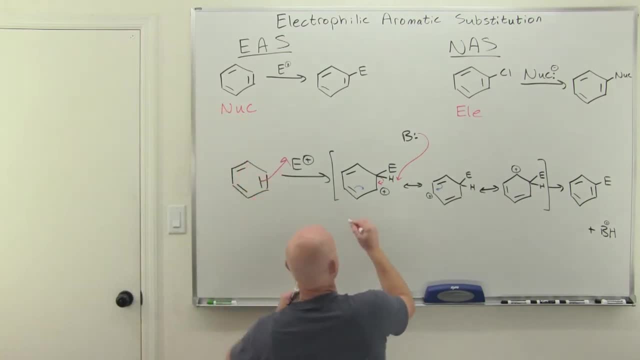 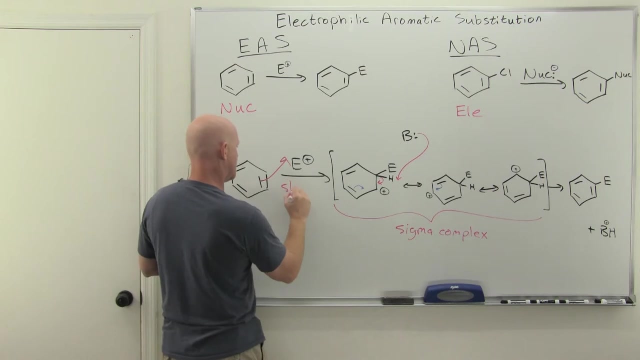 carbocation less stable. Now one thing to note: this lovely carbocation intermediate that is resonance stabilized gets a special name. It is often referred to as the sigma complex, So in your EAS reaction. So this first step is the slow step because we're definitely going from 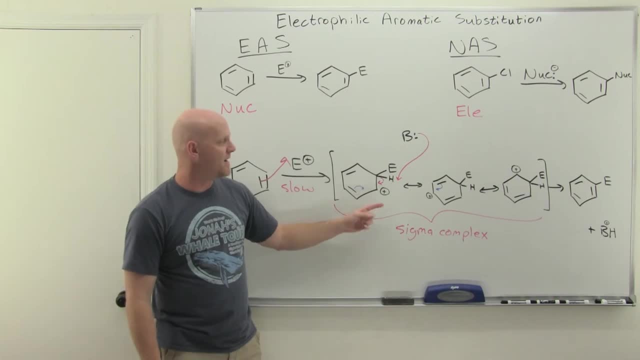 something that is aromatic. but this carbocation is not aromatic. Notice that carbon. right there is sp3 hybridized and you can't have any sp3s in the ring. Otherwise you don't have a continuous ring of overlapping p orbitals. So going from an aromatic reactant to 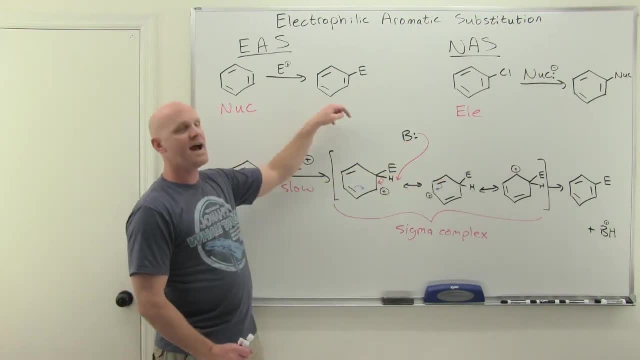 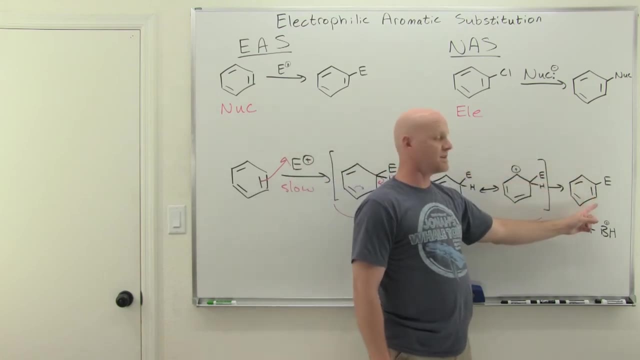 a non-aromatic intermediate going to have a very high activation energy for step number one. So that's our slow step And again, really advantageous then if we restore aromaticity to get our final product. And again that's why we do substitution instead of addition. 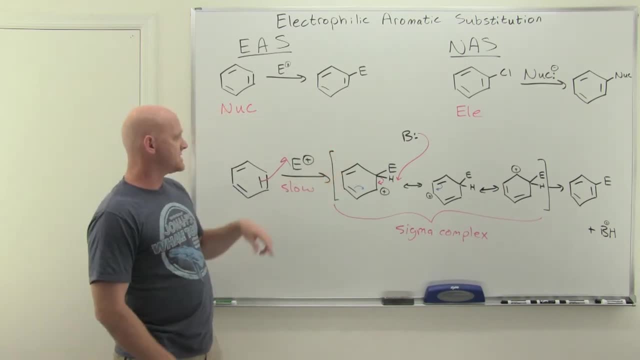 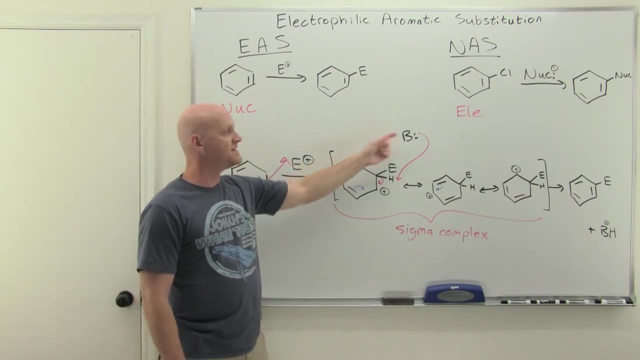 Cool. So this is kind of the generic mechanism. The blanks we'll have to fill in is: you know what's the electrophile for each of our individual EAS reactions and how is it generated, And then who's the identity of the base. but they're all going to follow this, the at least. 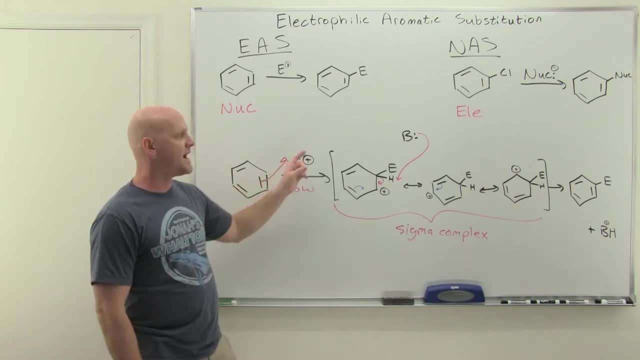 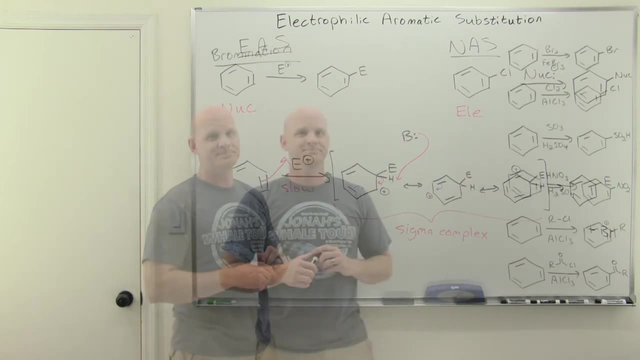 they'll finish off their EAS reactions with So nucleophilic attack followed by a proton transfer, just a deprotonation to restore aromaticity. Let's take a look at them individually, All right. So here are kind of our six fundamental EAS reactions We've got. 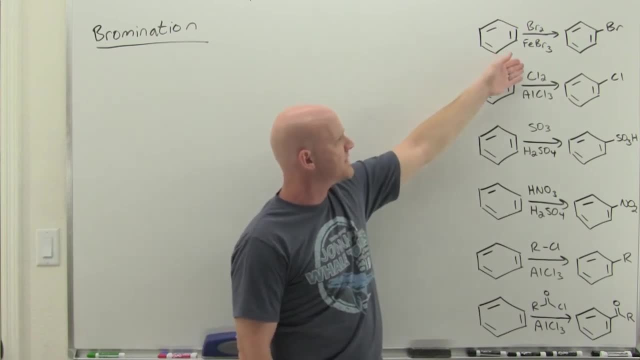 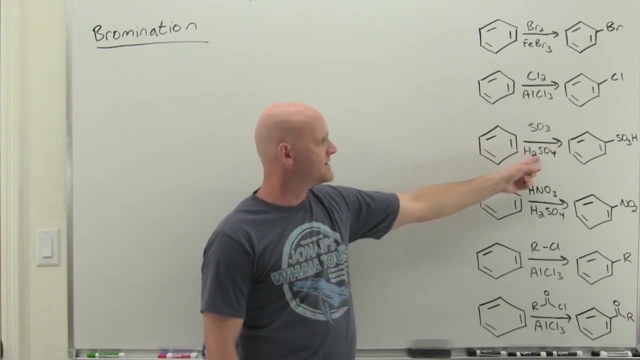 bromination with Br2FeBr3, chlorination with Cl2AlCl3, sulfonation- here with what we call fuming sulfuric acid, a combination of sulfur trioxide and concentrated H2SO4, nitration with what we call mixed acid, which is a mixture of nitric acid and sulfuric 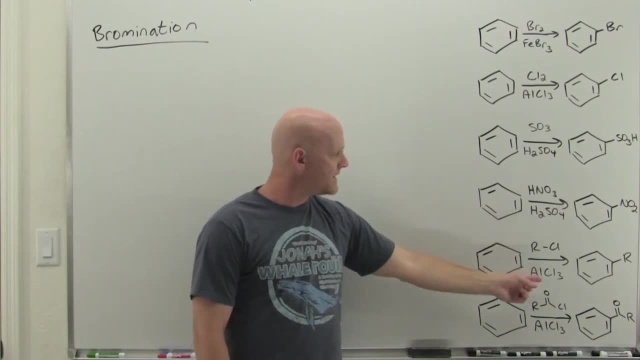 acid, Friedel-Crafts alkylation, where you've got an alkyl halide and aluminum chloride, And then finally Friedel-Crafts acylation- And that carbonyl group is called an acyl group here- where we form a ketone or, in one special case, an aldehyde on your benzene ring. So we're going. 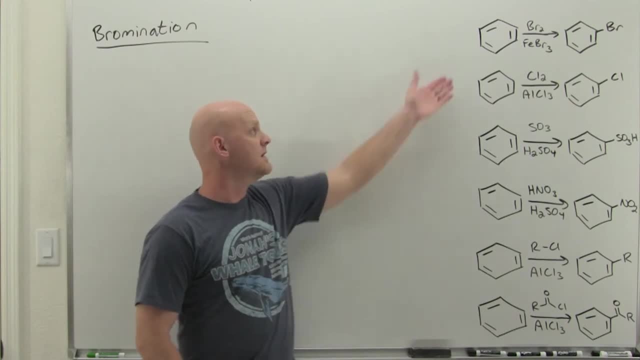 to cover these in sequence and go through the mechanism of all six of these. So start with bromination here. And we said before that if you just do this with Br2, it generally is not going to work. in most cases You need this FeBr3 and this FeBr3 functions. 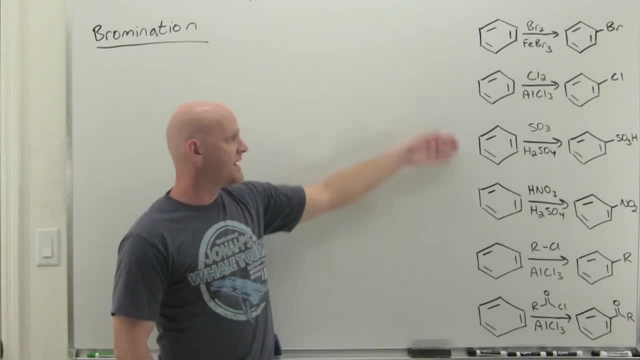 this is what we call a Lewis acid catalyst, And we're going to find out that all of these are going to be catalyzed by some sort of acid, most of the time with a Lewis acid, which is typically a metal ion like iron or aluminum, as we see in a lot of the cases here. So, but these other two? 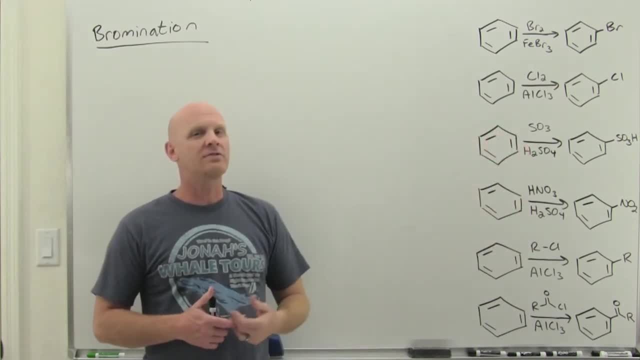 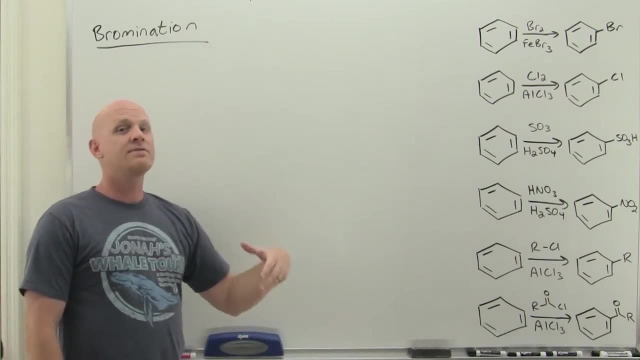 here are actually catalyzed by sulfuric acid instead. So but we're going to have some acid catalysis going on in most of these in one way, shape or form. So we said earlier as well that you've got to form your electrophile in every one of these cases in C2 before it can react with the 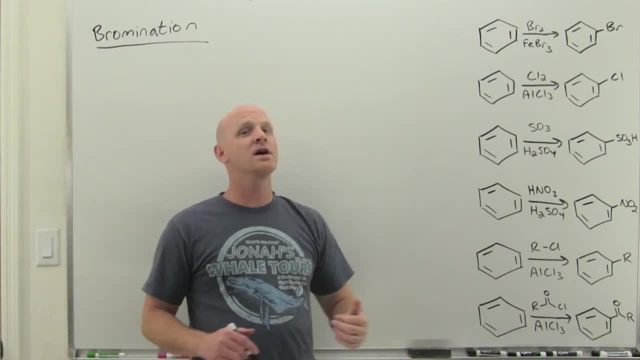 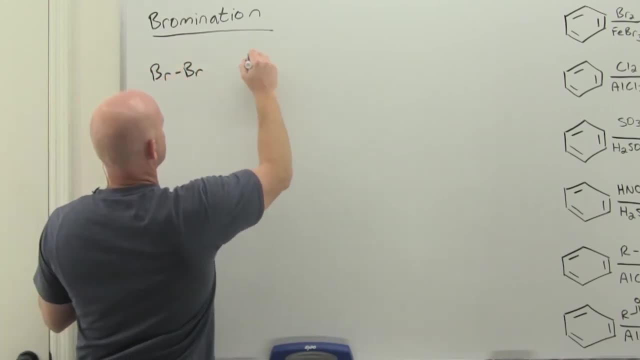 benzene. So because it turns out like Br2 itself, it's not a good enough electrophile. We need something more reactive, And so before we can get benzene involved, we first got to form our electrophile. And so what happens first? here is one of the bromines in Br2 is just going to attach. 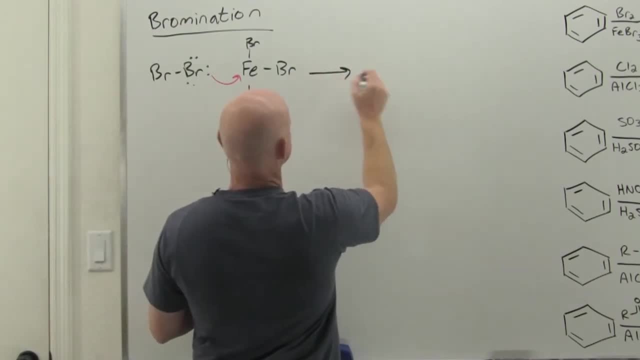 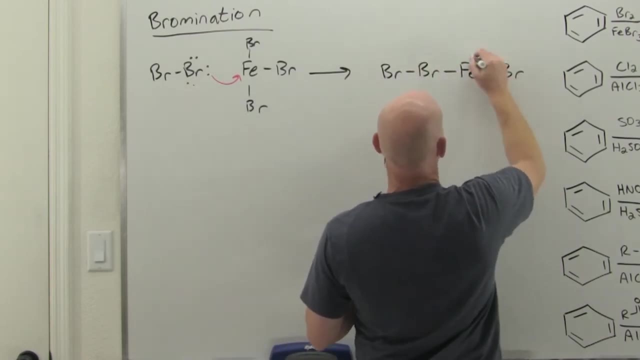 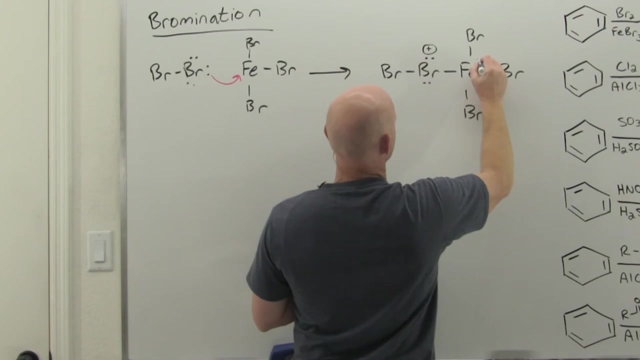 to iron. That is actually step one here. Well, when this happens, you're going to leave one of your bromines positively charged, and then the metal ion will be negatively charged here. So- and in this case it turns out, it's actually 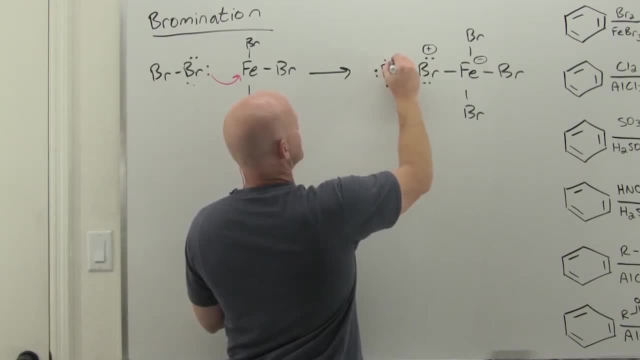 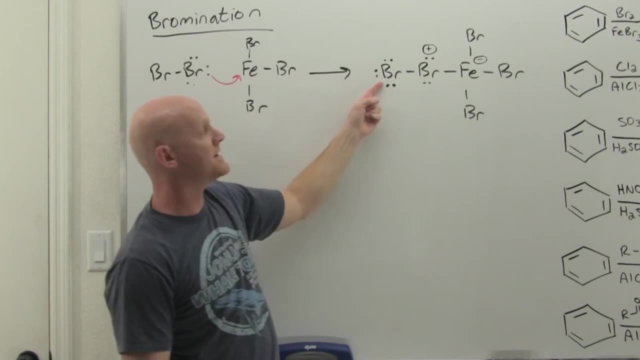 this bromine on the end and I'll draw his lone pairs in. So that actually is now also partially positive due to the positive formal charge of the bromine exome. It's pulling electron density away from making him partially positive And it turns out he's the electrophilic species, He's the one. 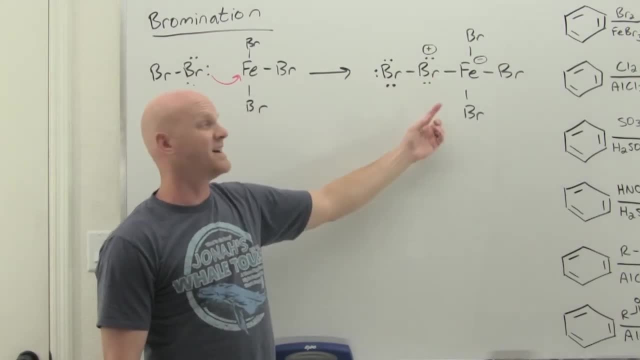 we're going to attach to. So we're going to leave one of the bromines in Br2 and we're going to. You might be like, well, why don't we attach to the positive one, Chad? Well, again he's got more. 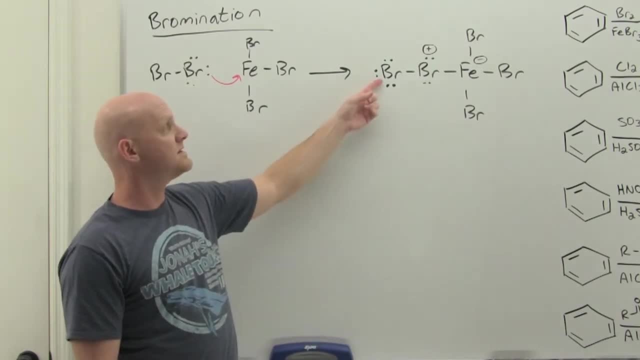 bonds than normal already. We don't want to make any more new ones to him. It's this guy we actually want to make the bond to, as it turns out, So let's see the way this works. So for now, we've got our. 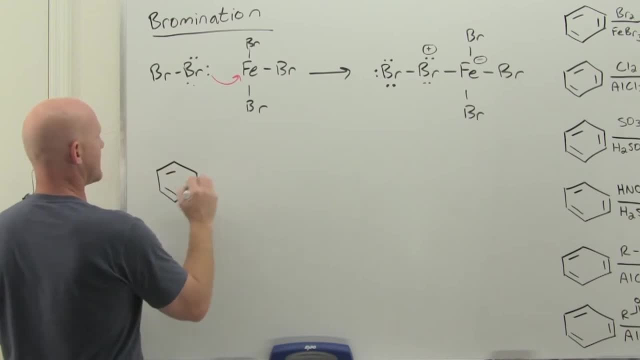 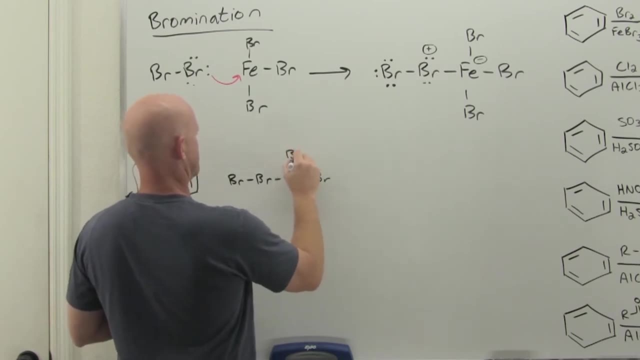 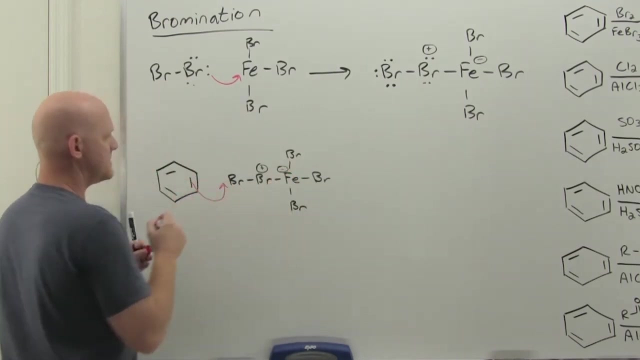 benzene going to get involved. We've now shown the formation of our electrophile, And so now benzene is going to come and attack that again, outermost bromine, So that bond to the other bromine breaks. So and now we've attached and formed our carbocation. 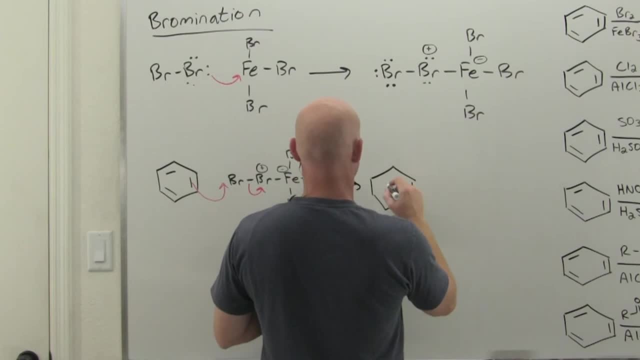 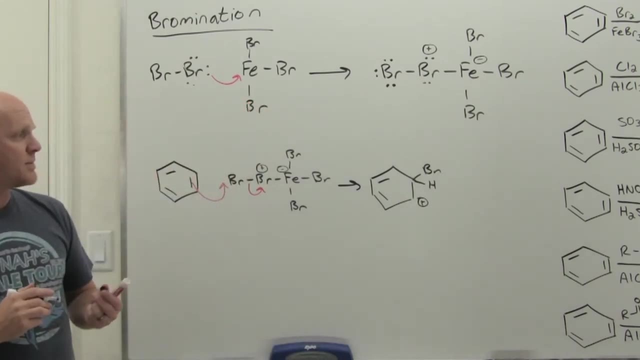 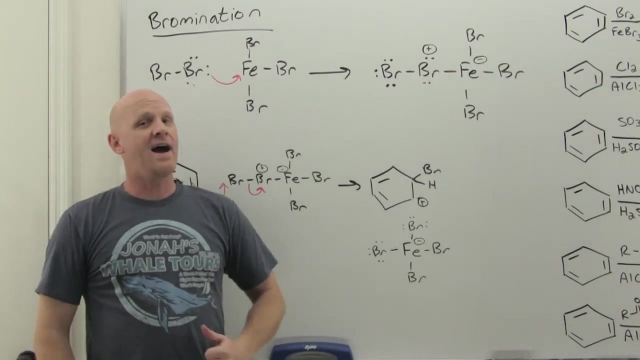 We've got a resident stabilized carbocation form. We've also got FeBr4 that will be in there as well, All right. So we've got this resident stabilized carbocation that we're always going to have. And in doing the mechanisms of each individual reaction, I'm going to avoid drawing all the 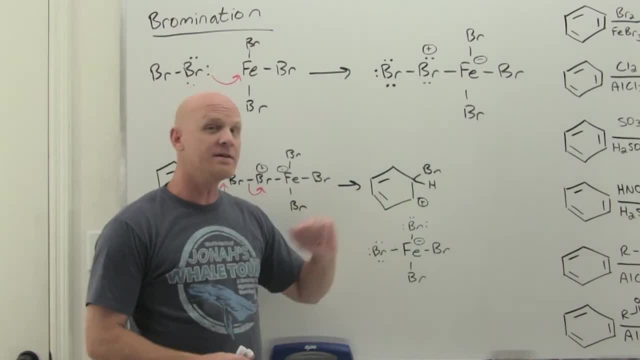 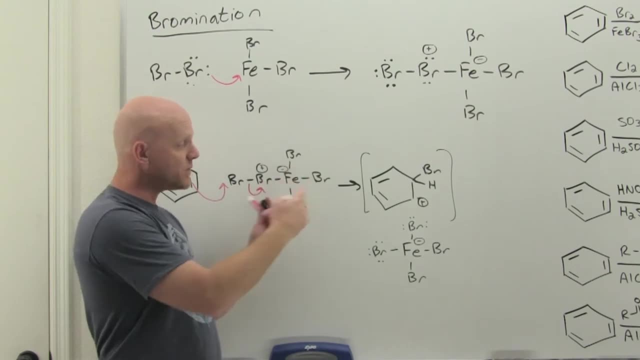 resident structures for the sigma complex, simply because it's just going to be repetitive and not function a lot. But again, every time you're going to have a resident stabilized carbocation, that would have three resident structures in every one of the reactions we're. 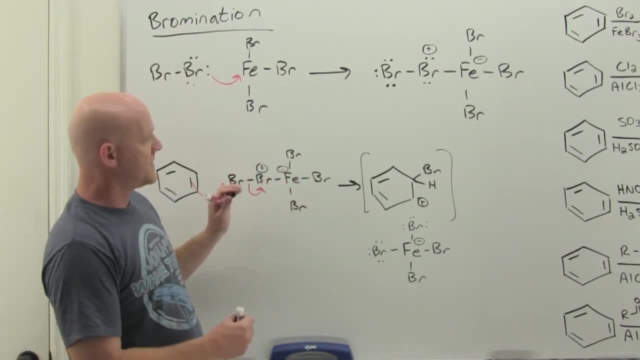 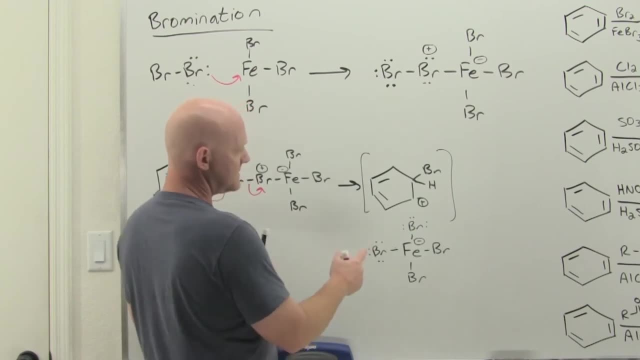 going to do the mechanism, for I'm just going to save some time here. So, but we've done that. We've done nucleophilic attack and formed our carbocation. We would draw resident structures as part of any formal mechanism. So, and then we need a base, And in this case the base is going. 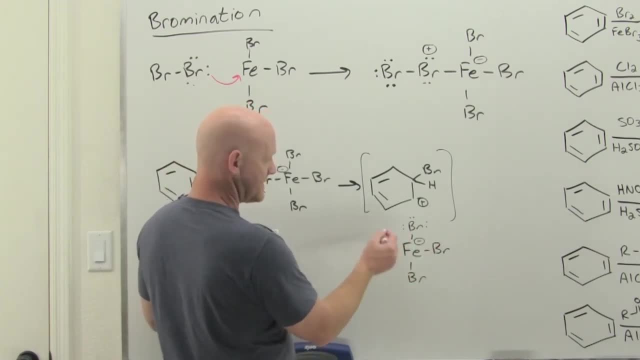 to be one of these bromines breaking off And technically it could be the one that you know attached right here back in this case, but technically it could be any of these in this case. but I'll make it that one, Why not? And we'll come back over here and he's going to come. 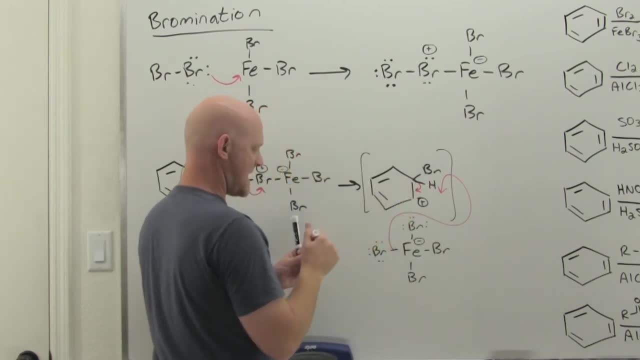 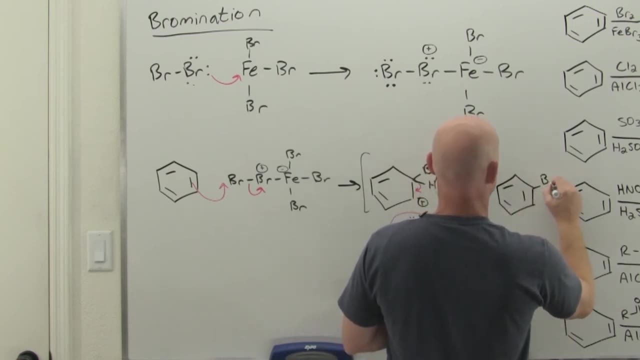 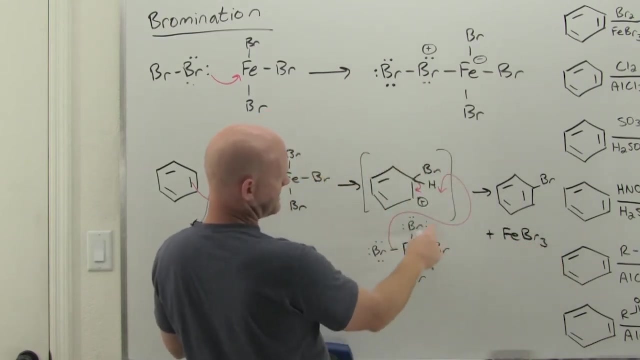 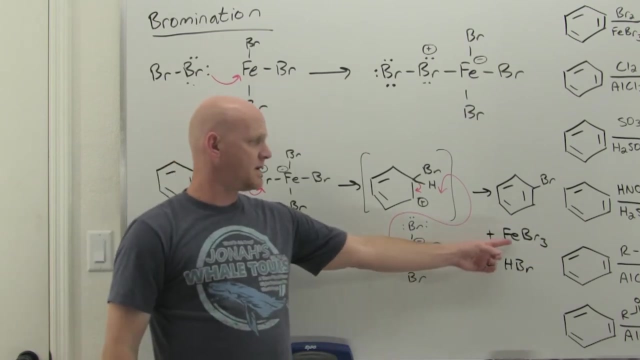 and deprotonate that hydrogen so that we can free up those electrons to reestablish aromaticity. And so now you're also going to form some FeBr3.. This goes back to being FeBr3, but we're also going to form some HBr here as well, And so, notice, your FeBr3 gets regenerated. 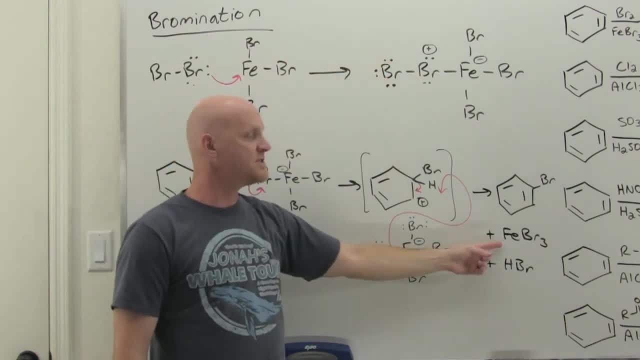 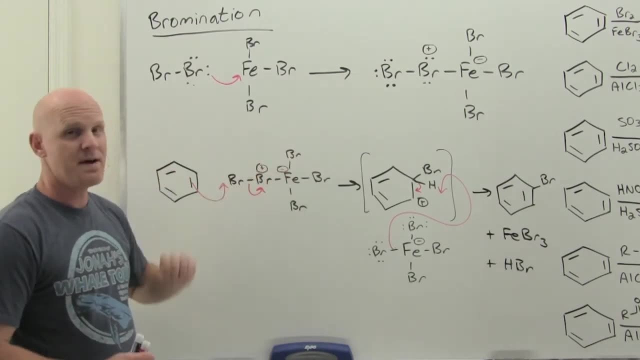 We used one of them way back at the very beginning to make our electrophile, but it gets regenerated before we're done, as should be true of any true catalyst. A catalyst is not consumed in the reaction, And this is the mechanism for bromination. Let's take a look and see. 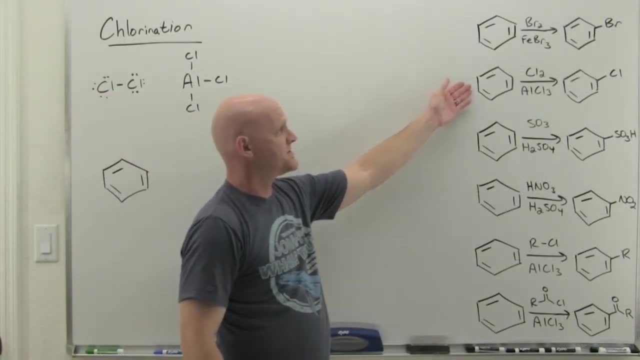 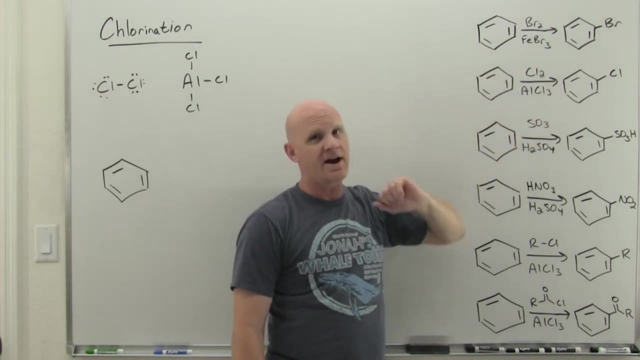 the similarities with chlorine. All right, So with chlorination. here we see we've got Cl2 and AlCl3.. This could also be FeCl3.. We can still use iron here as well, just like we use an iron Lewis acid catalyst. 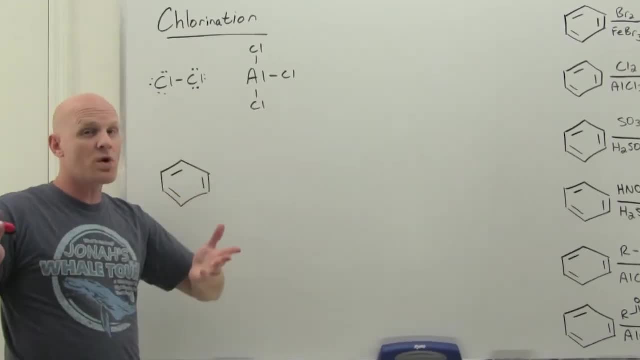 and bromination Works with chlorination as well, So but AlCl3 is used more commonly. but FeCl3 would work just fine. And first step again we've got to form our electrophile, And so, just like Br2 attached to FeBr3, we've now got Cl2 attaching to AlCl3. 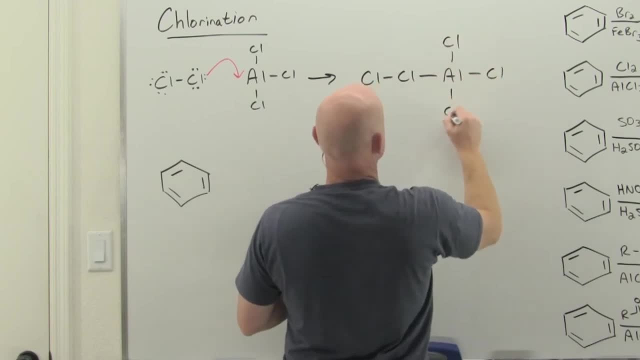 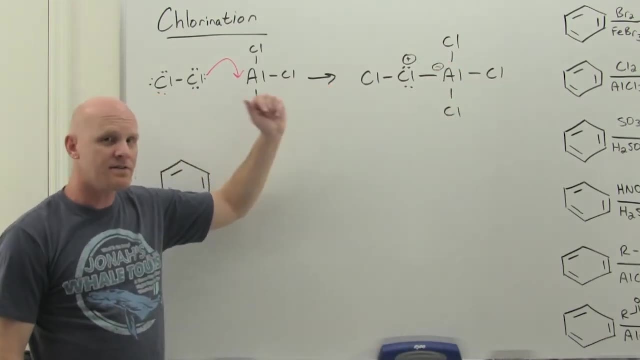 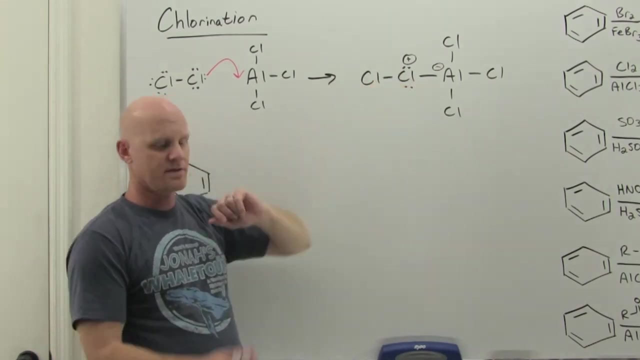 So, and once again it's actually this chlorine on the end that is the reactive one. as an electrophile, We're going to attach to him, freeing up these electrons to go back to that chlorine, so it doesn't have a positive formal charge anymore. So that is actually the species. 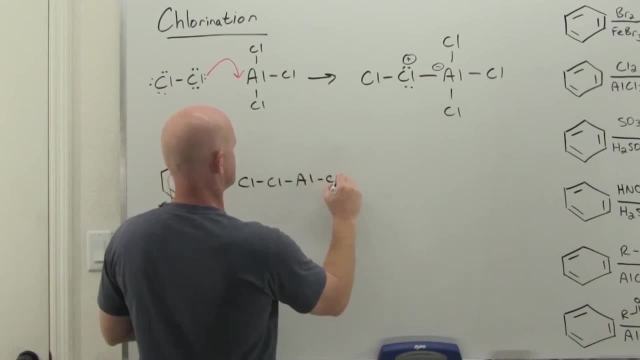 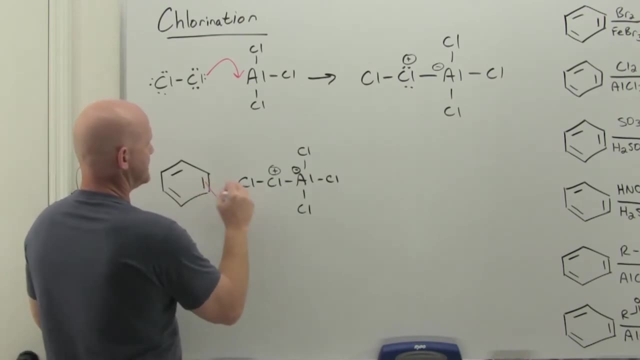 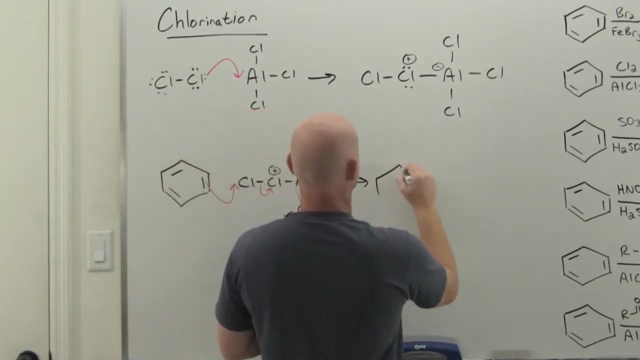 the electrophilic species that benzene will react with. So I'll do that. Okay, All right. All right, So we've got this benzene come and attach to chlorine and bond to the other. chlorine breaks. Well, we're not going to have that aromatic for a spell here. 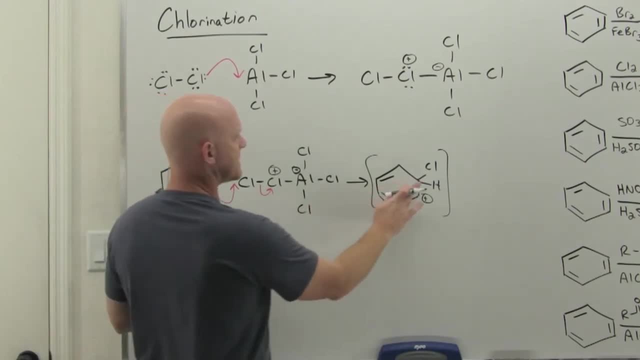 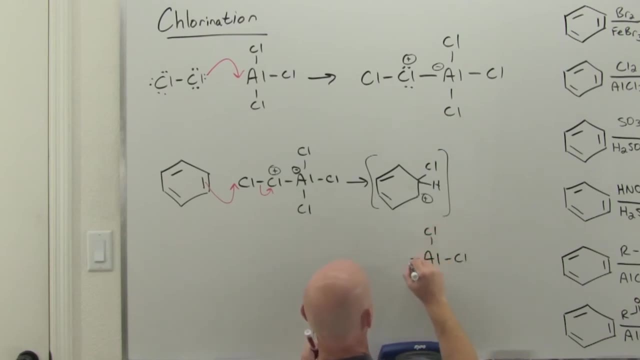 Once again, this would be a resonance stabilized carbocation. We're not going to draw out all those resonance structures And then we also form some AlCl4. And, just like in the last instance, one of these chlorines is going to break off instead. 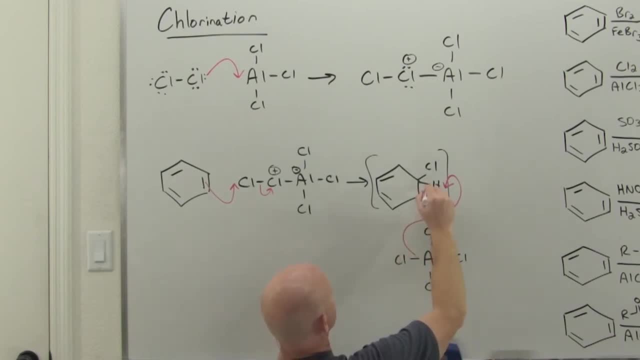 of a bromine. So and bond to that hydrogen that frees up these electrons to restore aromaticity. So we're also going to form some AlCl3.. We've regenerated our catalyst not consumed and then also formed some HCl as well. 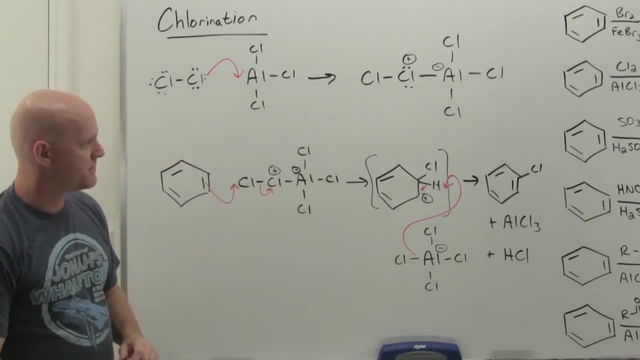 Cool. Exactly analogous to what we saw with bromine HCl. So free radical, I'm not sorry, free radical. electrophilic aromatic substitution, chlorination- exactly analogous to electrophilic aromatic substitution for bromination. All right, 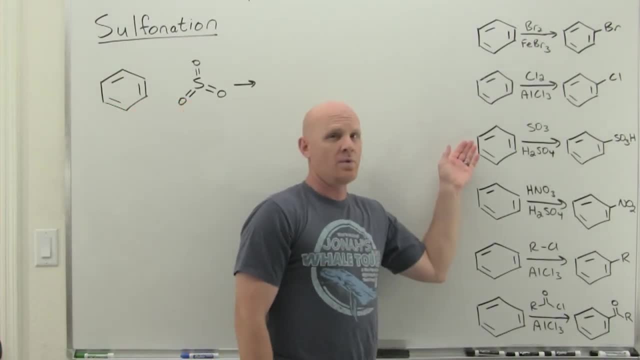 Now we're going to move on to sulfonation here and recall: the reagent is fuming sulfuric acid, a combination of sulfur trioxide and concentrated sulfuric acid. Now, one thing you should note is: out of all of these, this is the one reaction that ends. 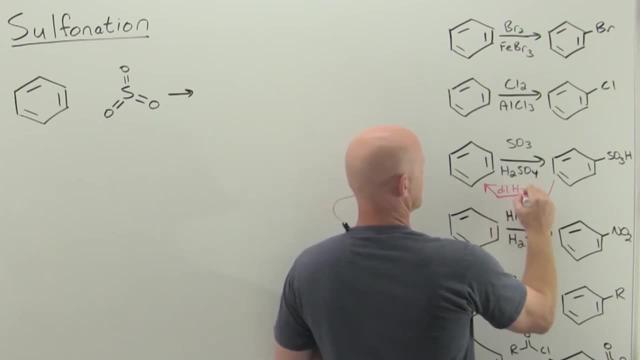 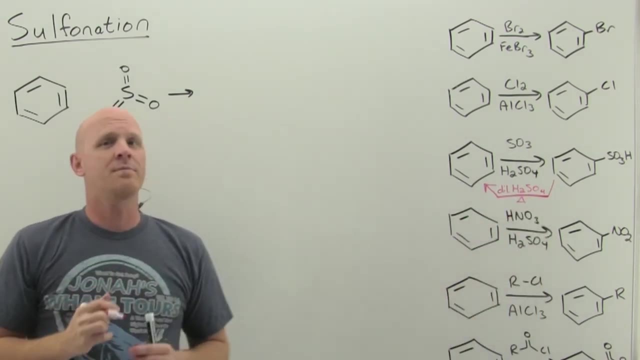 up being reversible And with dilute sulfuric acid. So, and some will actually show heat as well. So, with or without the heat is how it might be presented in your class, but it is reversible. With dilute sulfuric acid you can desulfonate as well. 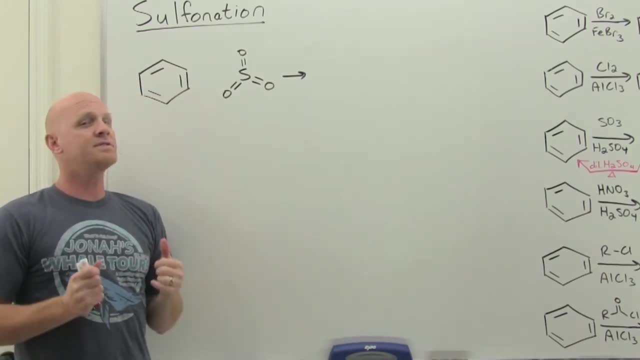 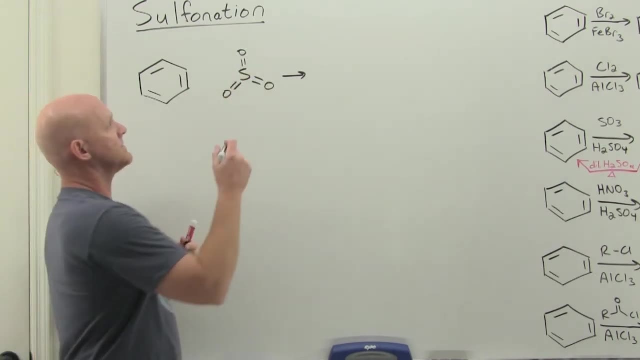 So let's take a look at the mechanism here. So in this case, most commonly this is actually the one reaction presented with a ready-made electrophile, So sulfur trioxide. some will show it actually as being protonated right off the bat. 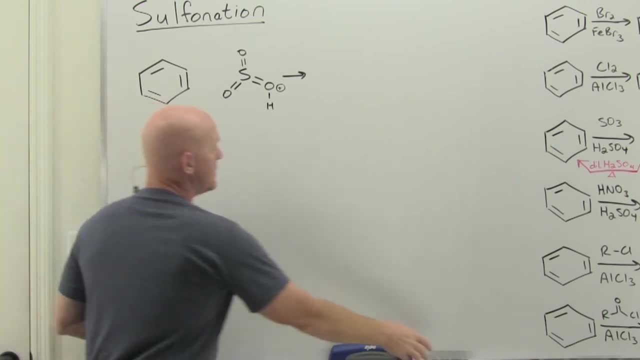 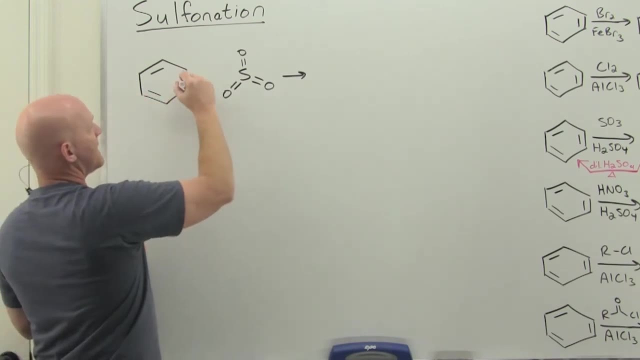 So you'll have to protonate it first from the sulfuric acid. But most textbooks actually show it just as the electrophilic species being the sulfur trioxide itself. And so we'll do nucleophilic attack on the sulfur here. kick electrons out to any one. 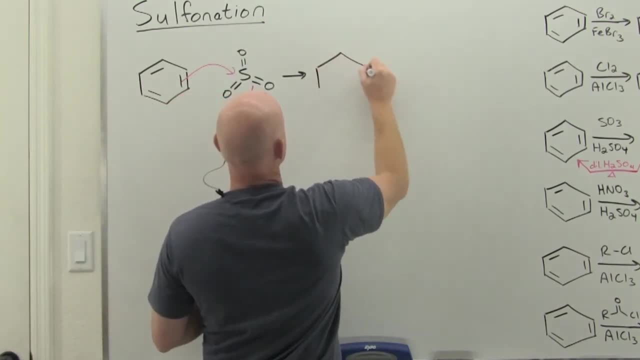 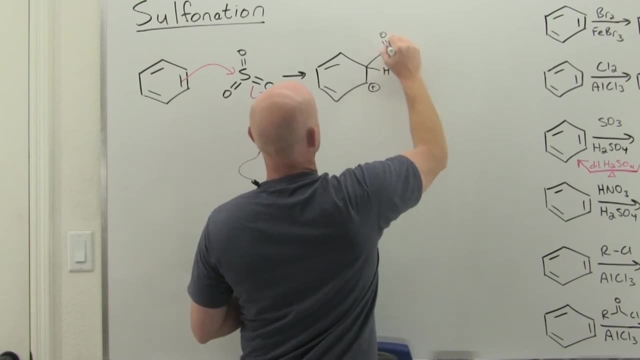 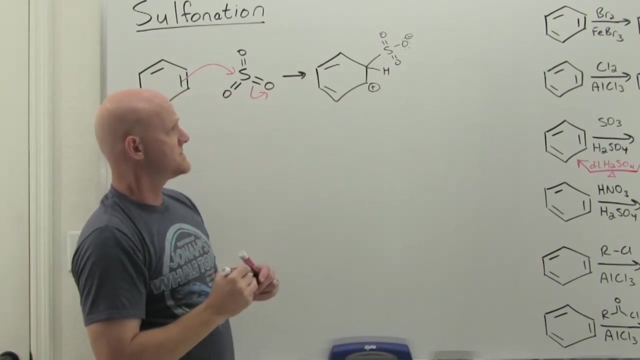 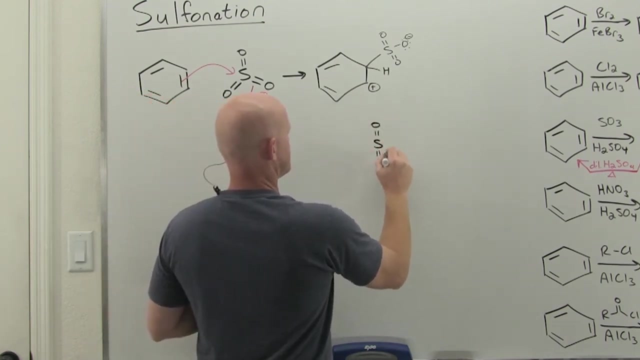 of these oxygens, Cool. And then we just simply need to Need to deprotonate this hydrogen, And our base in this case is going to be the conjugate base of sulfuric acid, So bisulfate here. That'll free up these electrons to restore aromaticity yet again. 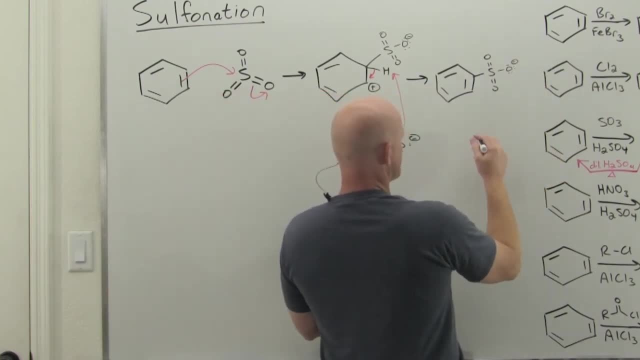 So and then from here we just form some sulfuric acid here, and there's solutions chock full of concentrated sulfuric acid. So even if we didn't, we'd have a bunch of it anyways. So and then we'll just deprotonate one of these sulfuric acids to protonate this guy. 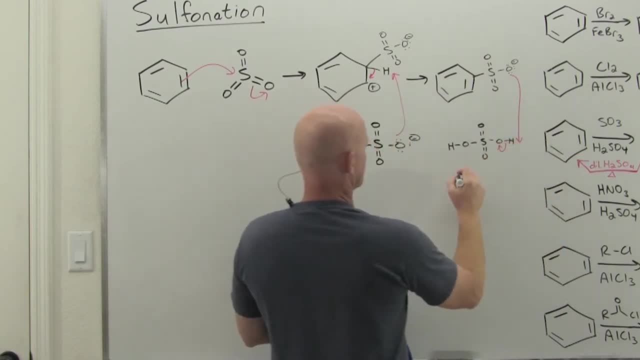 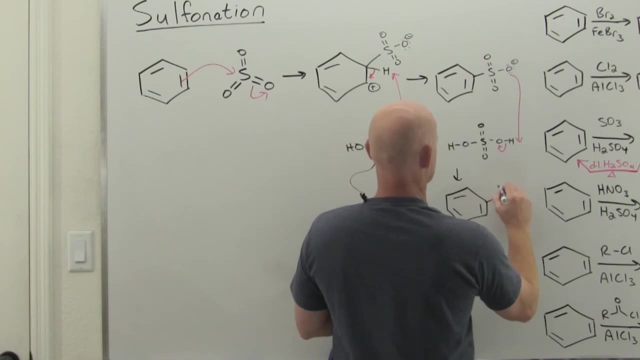 and form our sulfonate group, our sulfonic acid group, if you will Cool. And this right here is what we abbreviate as the SO3H group. So whether you've seen it drawn out the sulfonic acid group, or just see it drawn as SO3H, 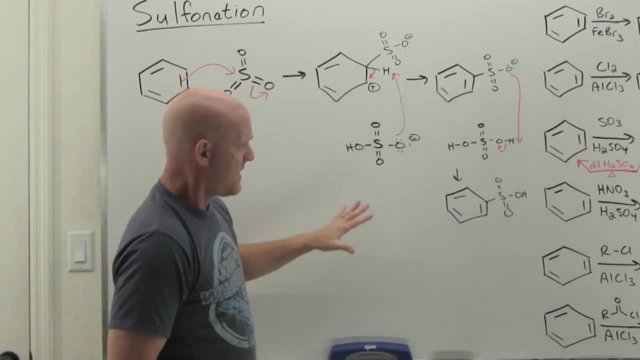 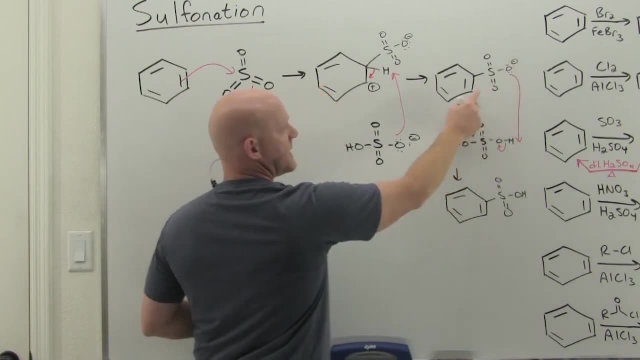 you should be prepared to see it both ways. All right Now if you look at the actual reverse reaction here. so from this guy we'd simply just go backwards and deprotonate And I'll pick up the mechanism from that guy right there. 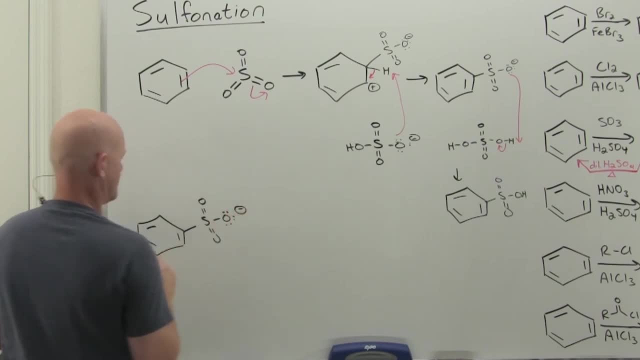 So, and in this case, when dilute sulfuric acid, we're going to have a fair amount of hydronium around. Some mechanisms show this as just H plus, So it'll actually show us the most likely source of that. 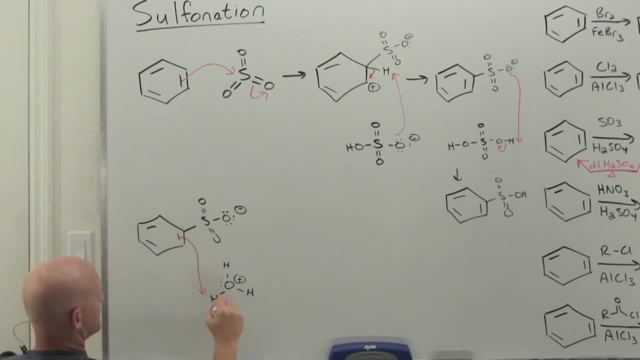 And that's the H3O plus the hydronium here, And we're just going to simply protonate. So this guy, Now we've added that H, right there Still have a carbocation here. So and then from here we'll kind of undo exactly what we did when we attacked the sulfur. 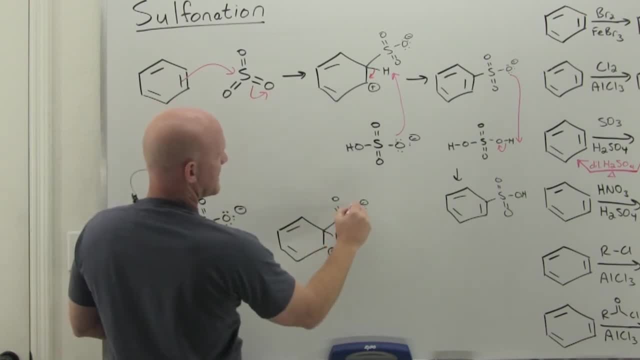 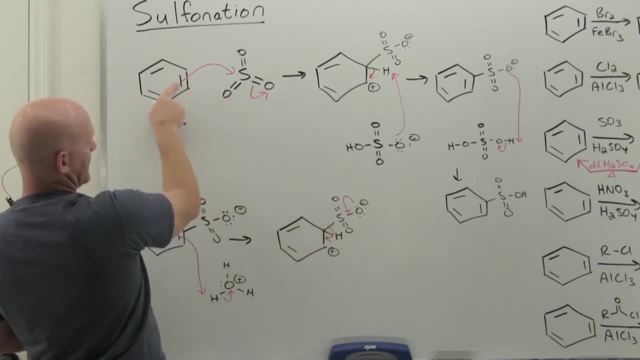 tracts to begin with, kick these electrons out to the oxygen. Well, those electrons are going to come right back in reform, a double bond to the sulfur, causing this to break off and leave and go back into being a pi bond. So exactly the reverse of essentially what we did in sulfonation. 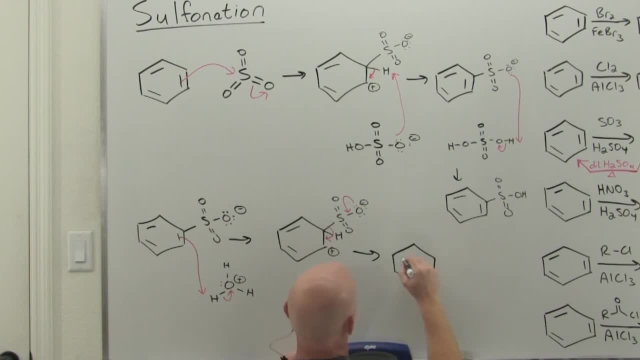 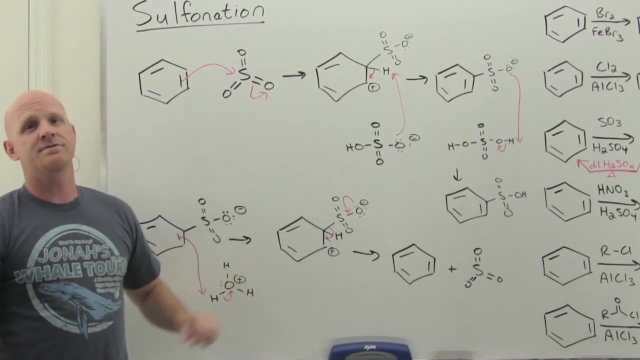 Cool, Cool, Cool. And we get back to having our SO3 and just plain old benzene. So cool, If they're going to leave something out, it is this desulfonation mechanism. So, but for some of you that would still have this presented in your course, we've covered. 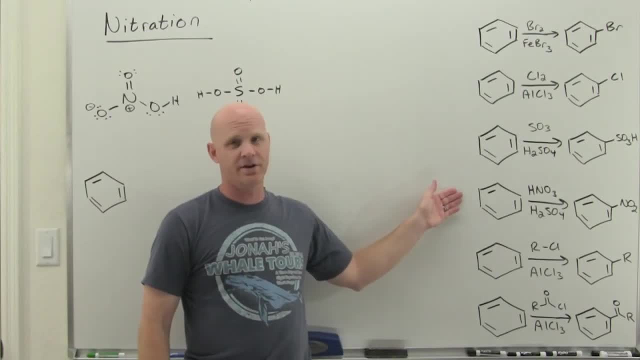 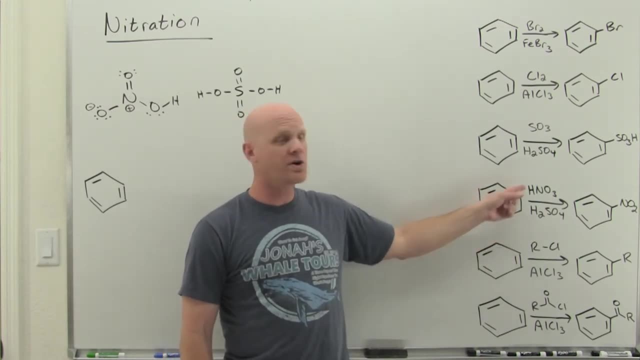 it here. So the next one we're going to look at is nitration. here And nitration, we use mixed acid as the reagent, which is a mixture of nitric and sulfuric acids. here And sulfuric is the stronger of the two acids. 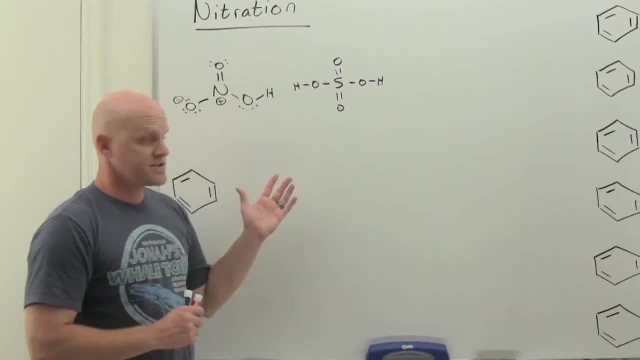 It's going to function as the catalyst in this case And, just like normal, we've got to generate the electrophile before we can react it with benzene, And so it turns out again sulfuric acid, nitric acid are going to react with each other. 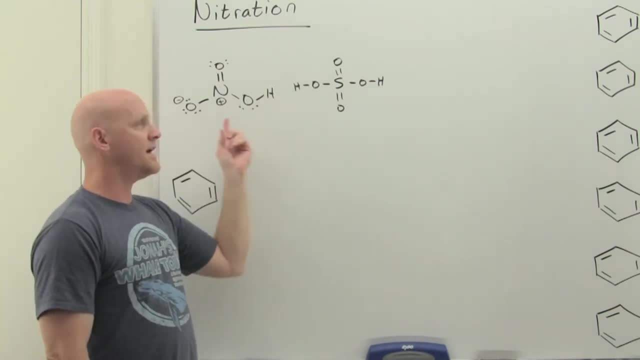 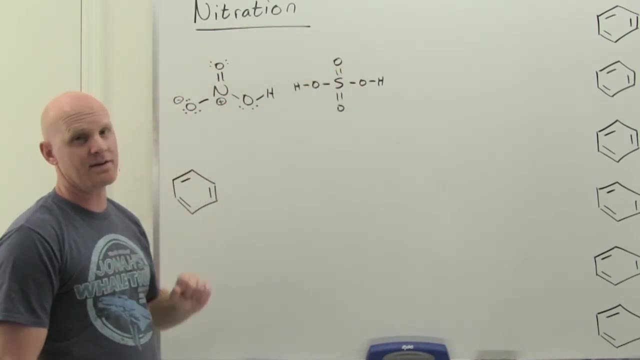 And with sulfuric acid being the stronger acid, what's going to be weird is that nitric acid, which is itself a strong acid, is actually going to act as a base, So sulfuric acid is actually going to protonate nitric acid. 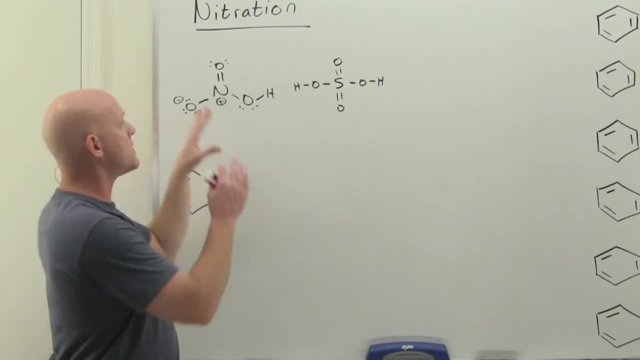 Now I usually ask my students in person: so where would be the most common place? you'd probably want to end up protonating the nitric acid here. So, and in this case, the highest energy electrons are on that side, The highest energy electrons are on that lovely auction. 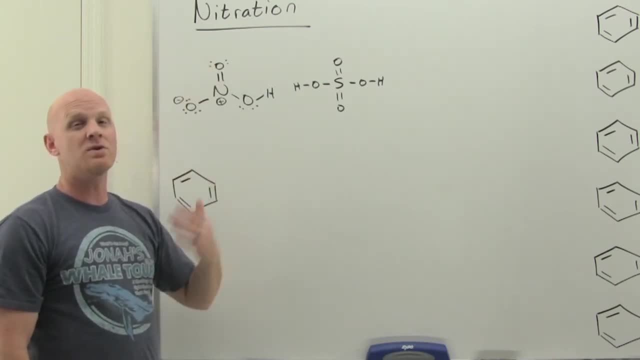 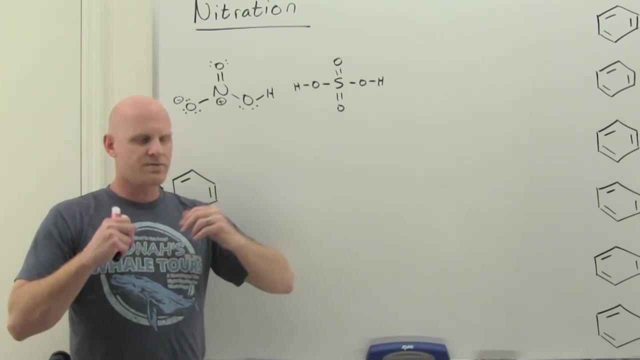 Technically it's shared between the two auctions. They get a negative charge And that would be the most likely place to get protonated. The problem is is it doesn't lead anywhere, And so kind of like if I invited you over for a party and I said, hey, I need you to. 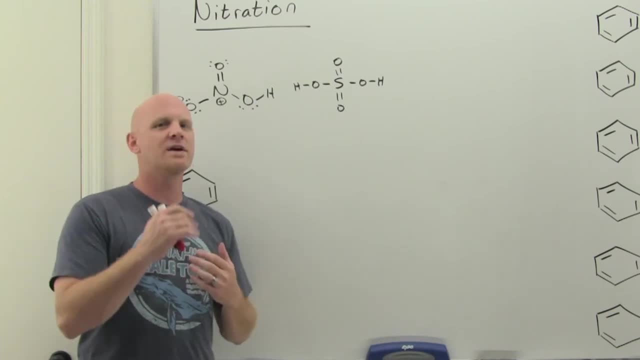 go get some ice And you're not familiar with my neighborhood, and so you're on your way to go get some ice and you turn into a cul-de-sac. Well, that doesn't lead you anywhere. So what would be the first thing you'd do right after turning into the cul-de-sac and 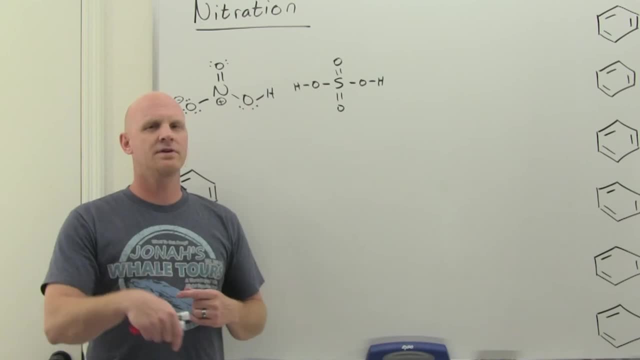 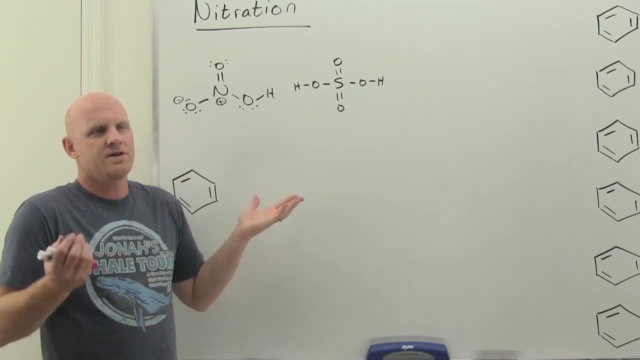 realizing it doesn't lead you anywhere. You'd make a U-turn and turn out, And so same thing here. If you end up protonating this auction right here, it doesn't lead anywhere, And so the only thing you could really do is then reverse course and unprotonate it. 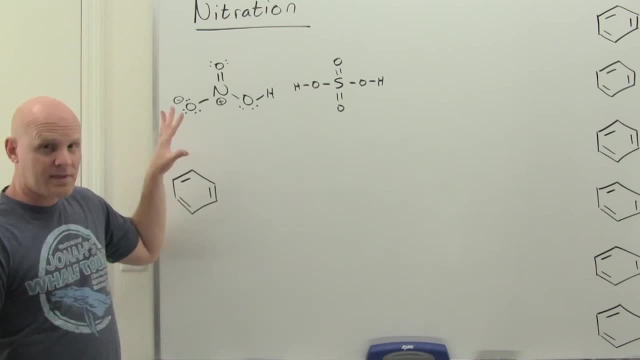 Or deprotonate it, I guess in this case. So it turns out. I'm only explaining that, because if you're wondering after the fact why we didn't protonate there, well, I mean again, it's the most likely place. 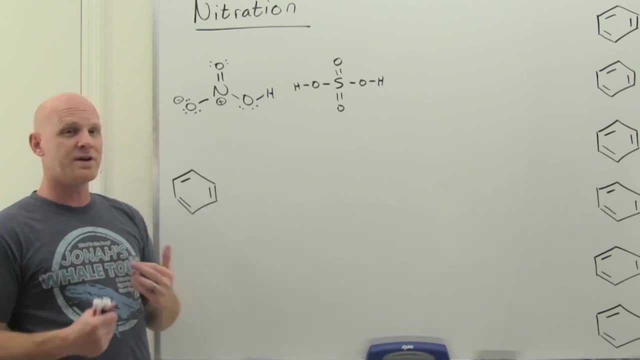 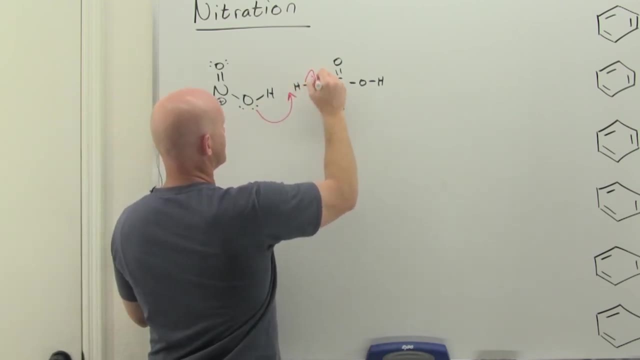 It probably happens all the time in the solution. It just doesn't lead anywhere, And so it's reversible and would come off, But we're going to end up protonating this oxygen over here instead, And again, it's not the most likely place to protonate. 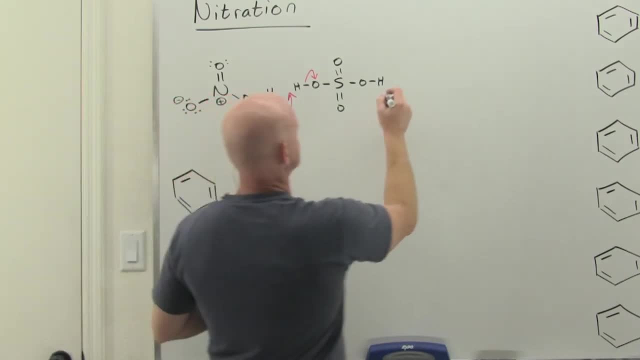 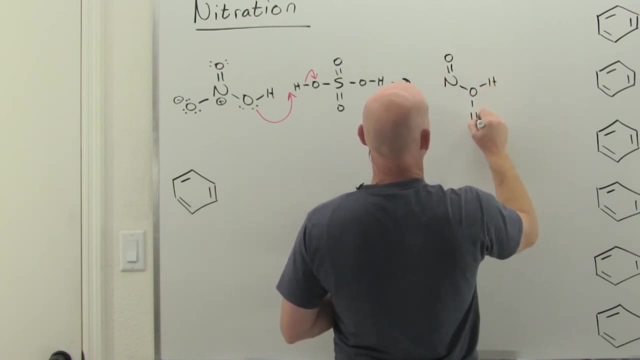 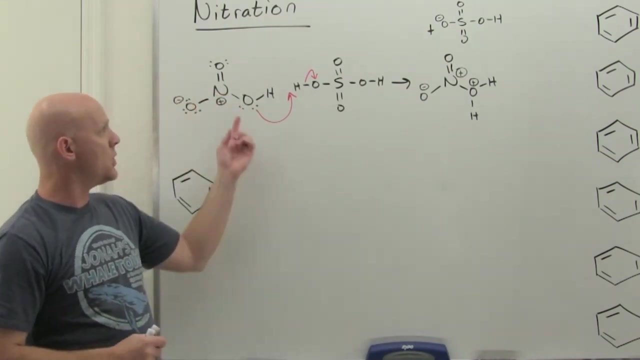 But it will. It will actually lead somewhere, All right. So we get this lovely species And it should look very familiar to what you did with an alkyl. Is an OH a good leaving group? No, it's not. How did you make the OH of an alcohol a good leaving group? 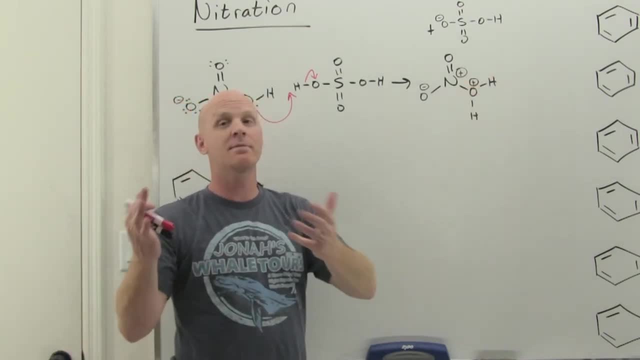 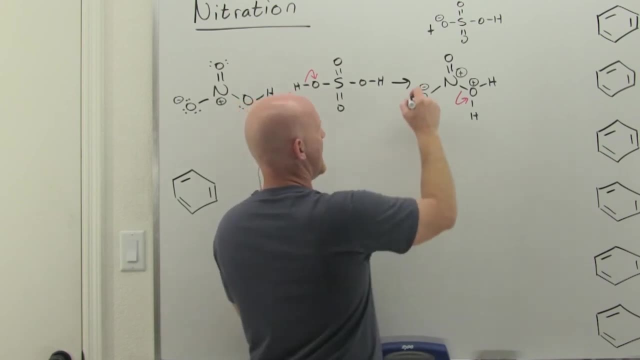 You protonated it And once it became water, it became a much better leaving group. And that's what's going to happen here, is it is actually going to leave. Now, that's not the only thing that's going to happen. It turns out simultaneously. we typically show pi- bond formation between the nitrogen. 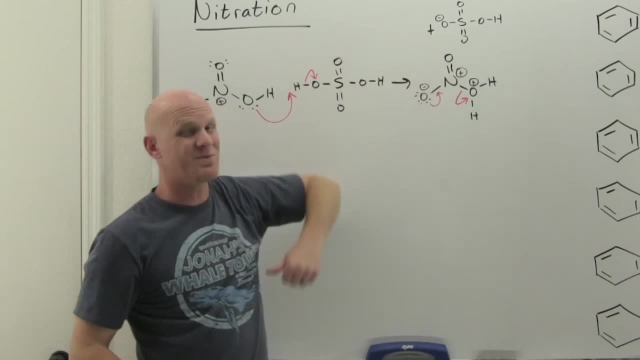 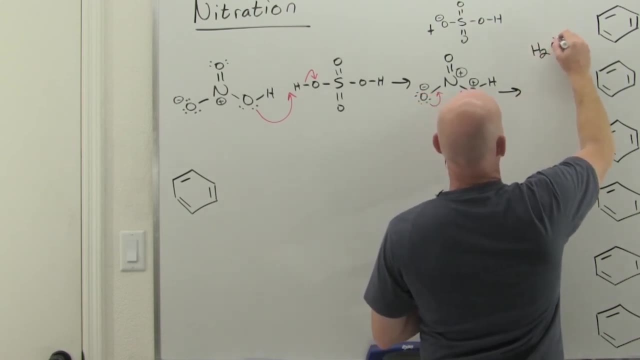 and oxygen there as well. That way we don't violate the octet rule on that nitrogen, which would be a really terrible resonance structure to draw Cool. And so in this case you are going to form some water when it leaves. 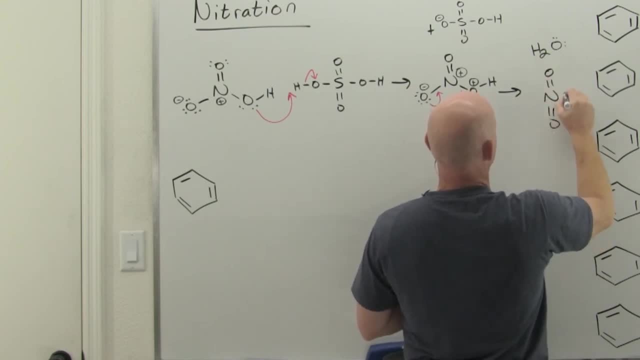 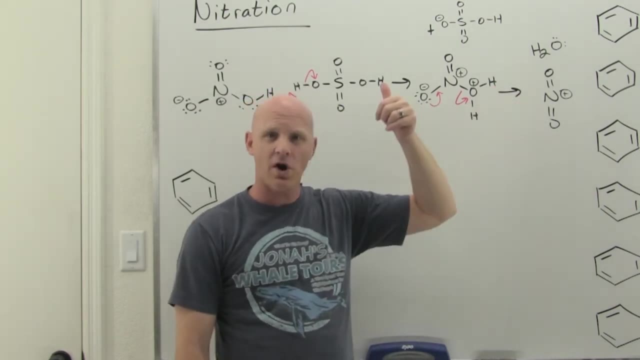 But you're also going to form this lovely species right here. So NO2 with a plus charge, And this is your electrophilic species, Again having a positive charge, great electrophile. That's what actually is now going to react with benzene here. 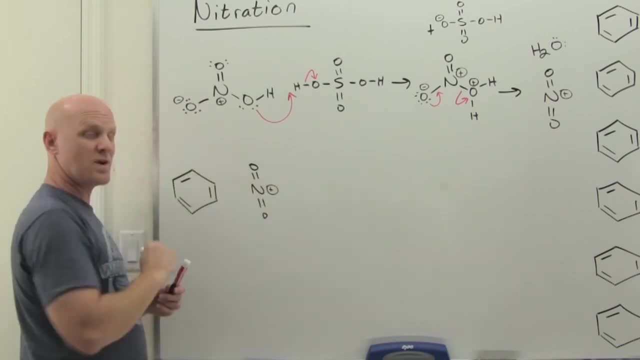 So two steps to form our electrophilic species in this one, And this is one of the more complicated ones that students struggle with a little bit. But it's just those two steps. You can relate it to what you did with alcohols: protonate the OH and then have it leave. 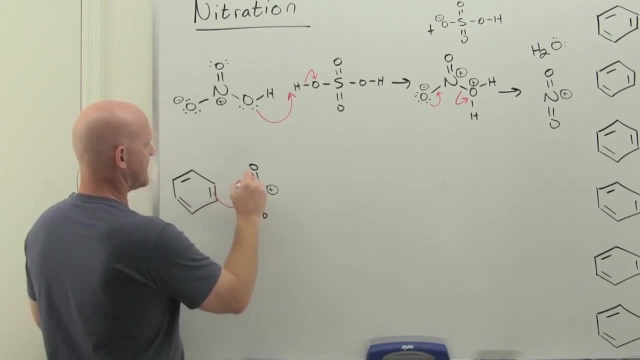 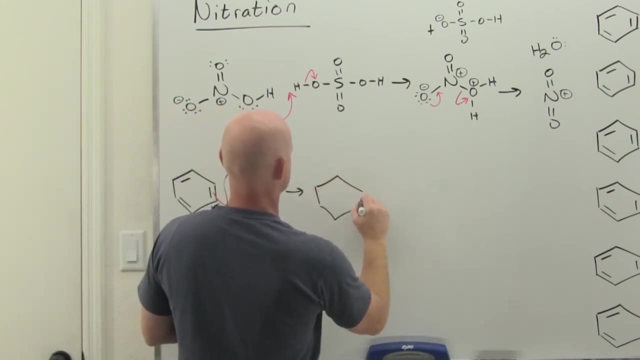 And there you go. All right, So we'll do nucleophilic attack. It doesn't matter which one of these auctions. we kick the electrons to, All right. We get our lovely carbocation And again, we typically draw this hydrogen because we're about to use it. 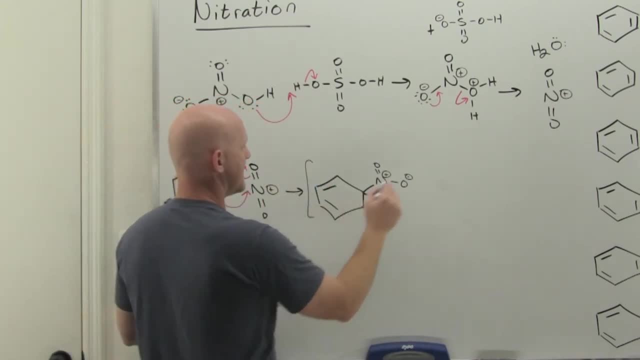 That hydrogen has been there the whole time, though This is also a resonance stable. This is also a resonance stabilized carbocation, But once again, I'm cheating and I'm not drawing all the resonance structures, But there would be three resonance structures.